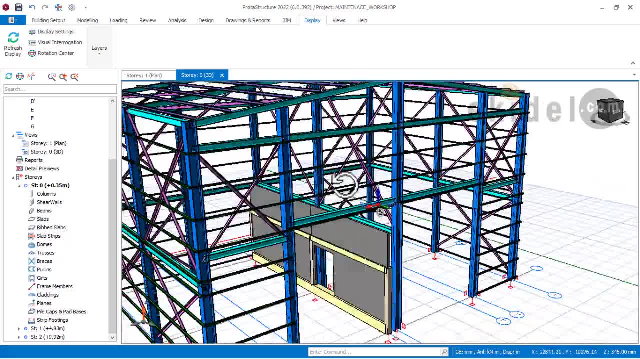 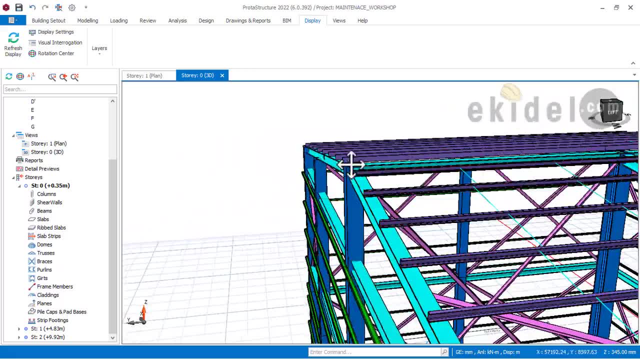 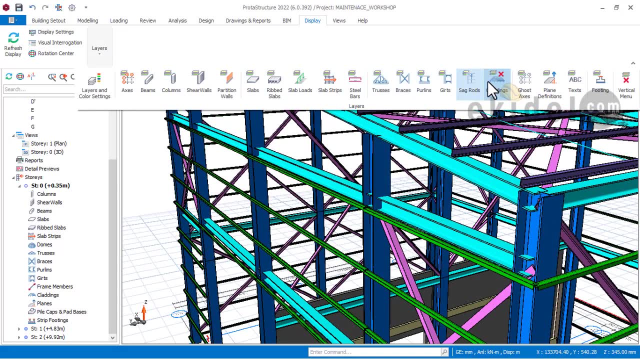 warehouse building and some other type of complex building in steel, you will begin to notice that you you might have a sloping, a sloping member, And in that kind of sloping member, if you are meant to add other components, you might want to develop a cladding, something like this here: 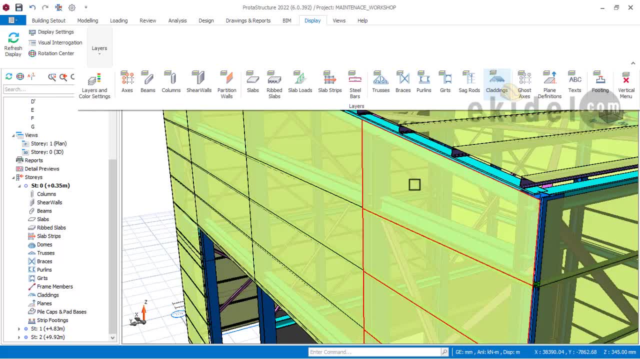 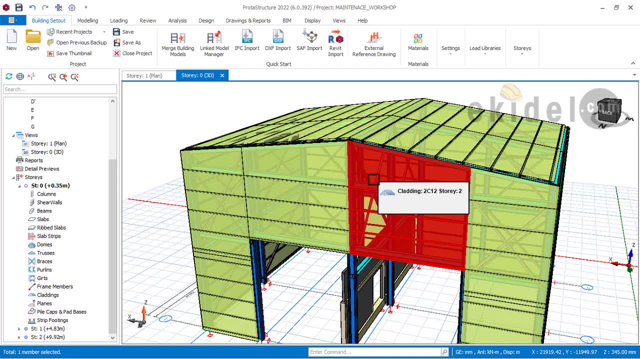 As you can see, if I turn on my cladding now, you will see that these claddings on this area they have sloping members, as you can see that. So I'll be showing you how to create your like a sloping cladding. 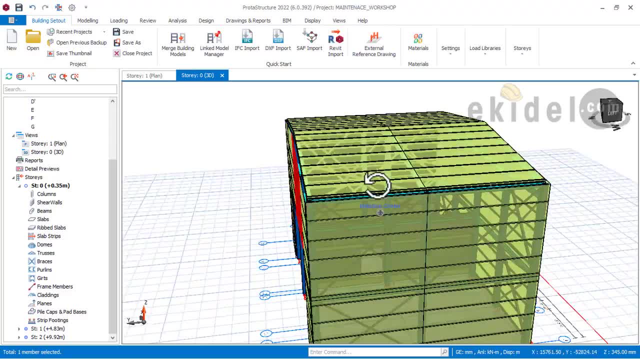 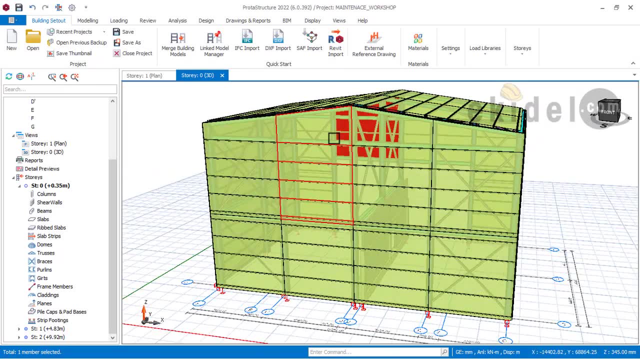 If maybe you want to put a cladding at an angle, I will show you how to do that. If you also look at this back here, you can see that most of the cladding here are all at an angle. So that is why I said this video basically is to show you how to create. 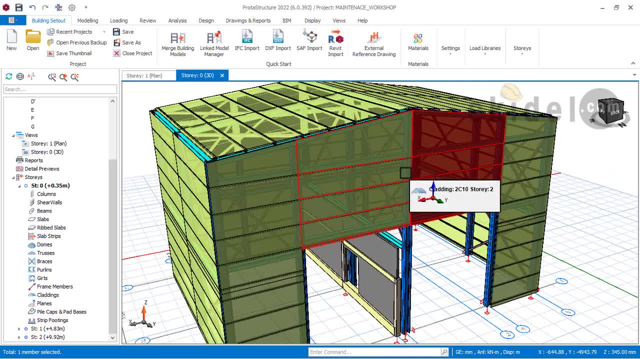 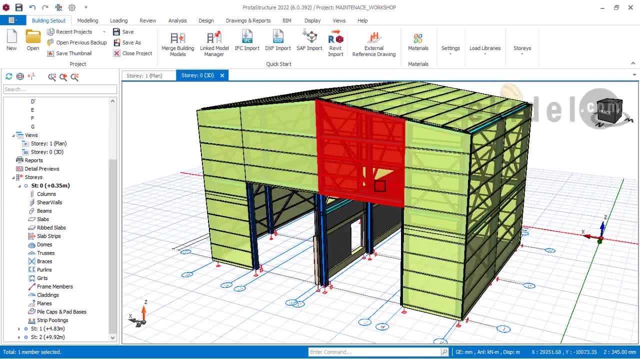 how to create an angular cladding. If maybe you want to slope the cladding in one particular angle, I'll be showing you that just now. Okay, so right now, let me just assume that we do not have cladding on everything here. 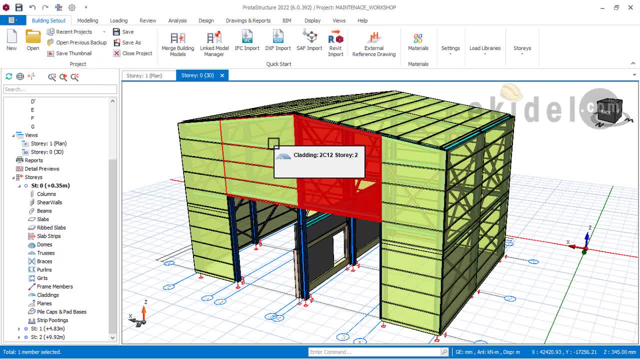 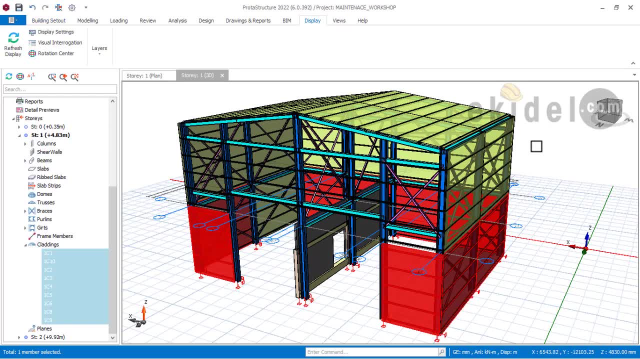 So I'll just take off all this cladding now and then begin to walk you through on how to create this cladding based on the angles. Okay so, okay, let's begin with that just now. Okay so, I'll just remove all this, my cladding here on my ground floor. 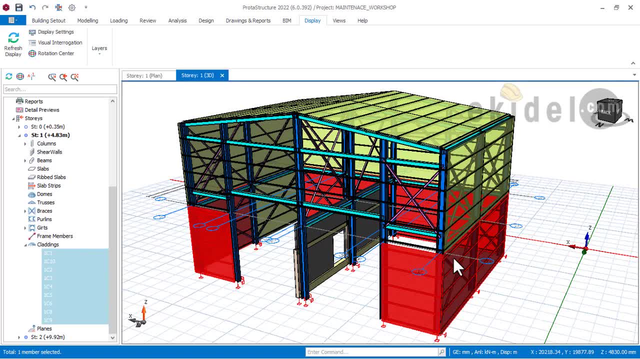 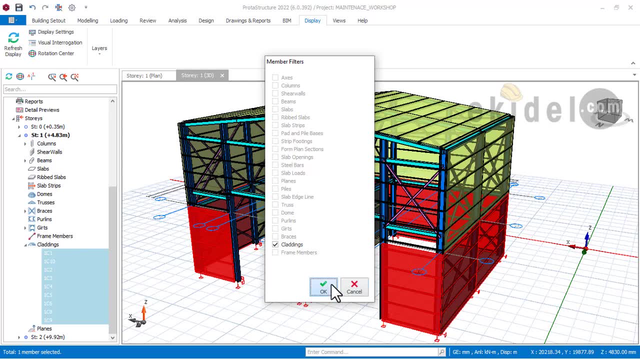 So I right click now and then say, delete Again. I'll still go, and then add up the cladding on the first floor. I'll just say, okay, yes, delete that. And then I'll also go again to my second floor here. 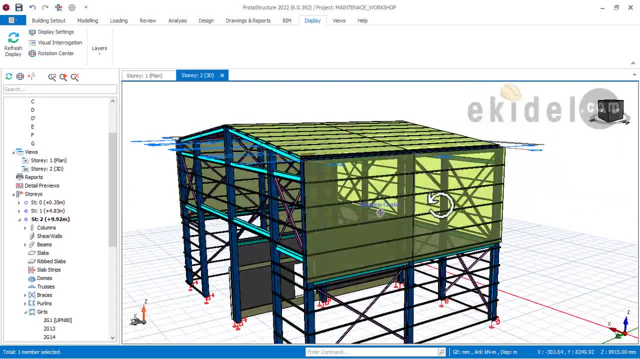 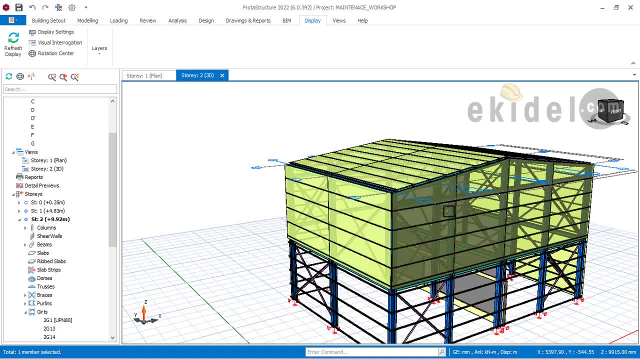 which is to remove the cladding at this level, because I have just removed all the cladding at the lower level, So at this level too, now I also need to remove all the cladding here. So to remove the cladding here. 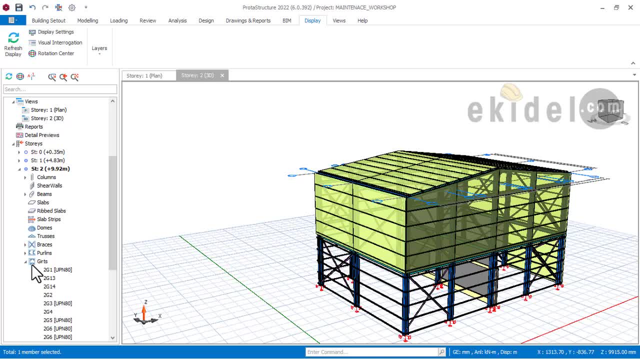 I'll just go here right now and I'll make story 2 active and then come to cladding under cladding of story 2.. This is story 2 here. yes, Then click on the first one, hold my shift key and then click on the last one. 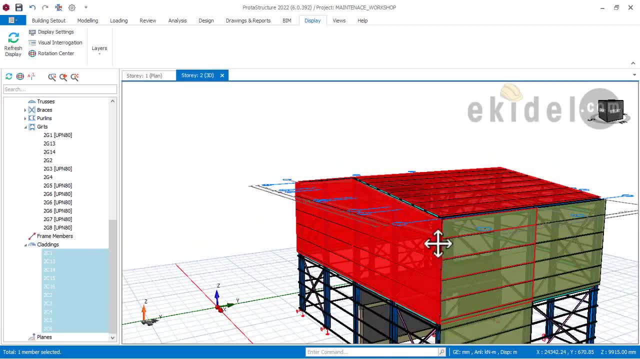 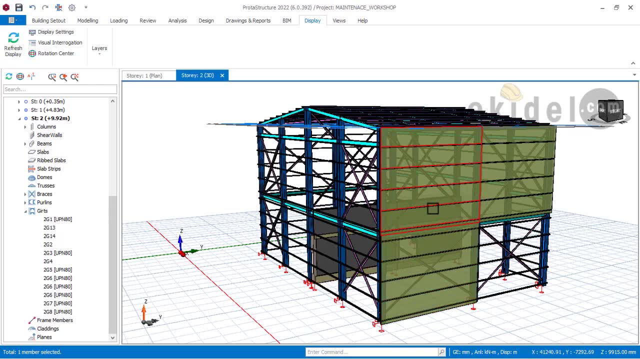 and it will just auto select everything of about the cladding, And then I'll just go ahead right now, right click and then say delete, Okay, that's fine. And then say okay On this other side- now I will click on this now again. 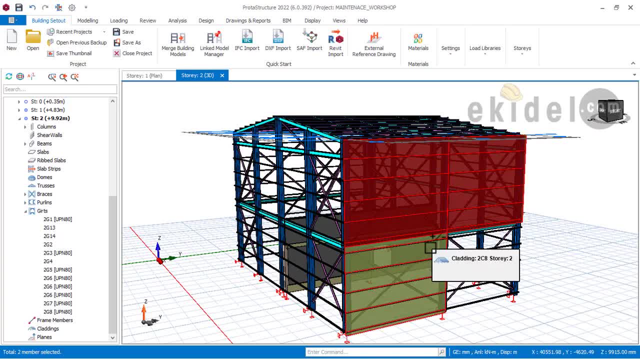 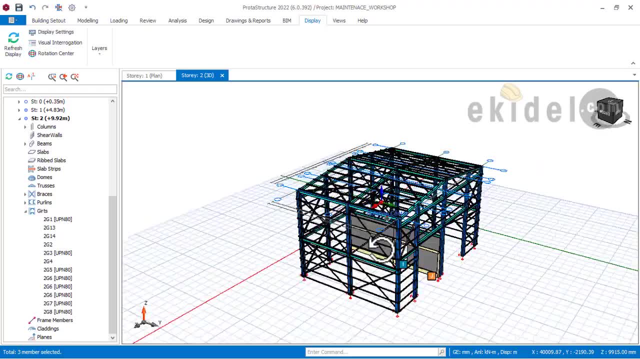 and then begin to remove this one manually here. By removing this, I remove this also. Okay, that's fine. And then just say delete, Okay. So basically now you can now see that we have all our steel, our steel members, being modelled. 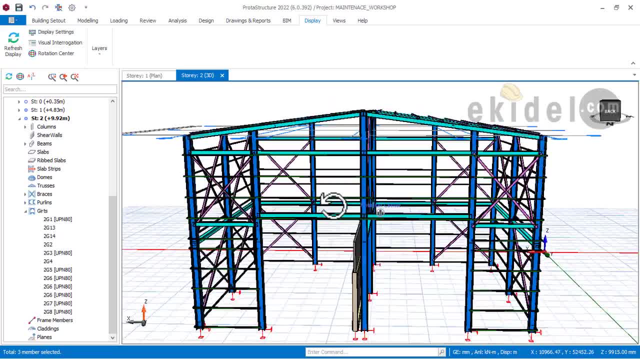 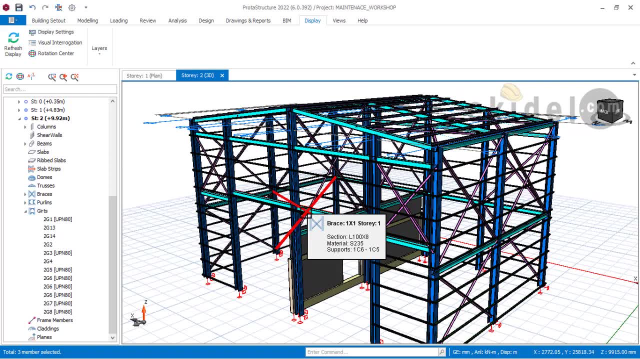 But right now, we now begin to input the cladding. So that is what I want you to see: how to input your cladding. Okay, so, first thing, to input our cladding, or to auto create our claddings in Kotatsu Twin Pins 2,. 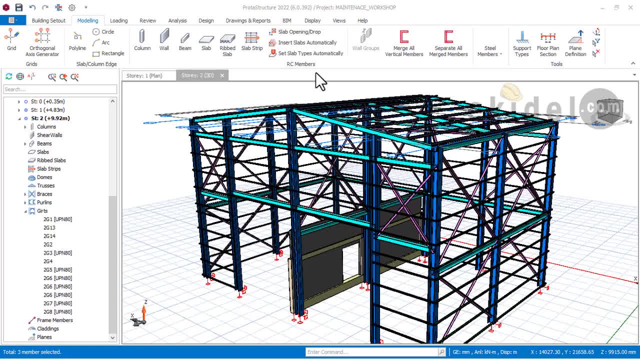 you have to go to modeling here, And on this modeling here the first thing you do is to have to locate this place here that says steel members, And then on these steel members- here there will be a drop down members- and then just locate cladding. 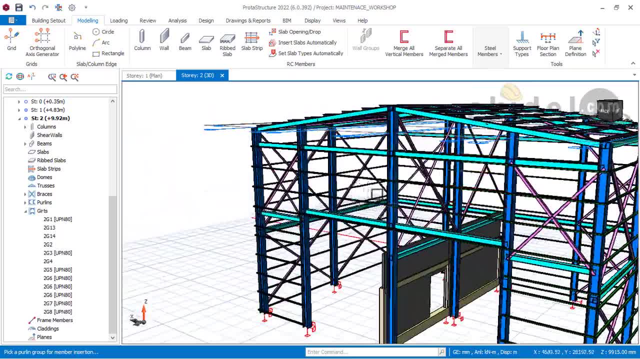 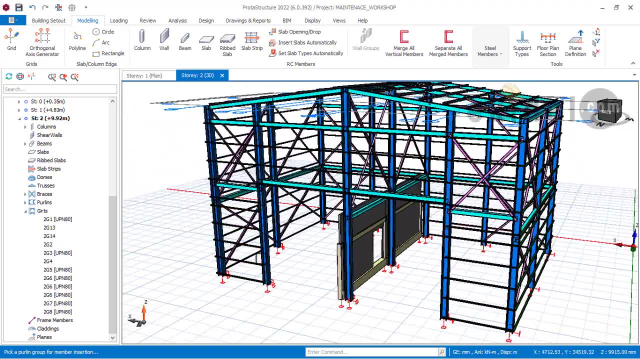 Now we have, we have done a course video on this steel, on this, on the full design of this steel model, where we use the CAD file and all that. Okay so, and if you, if you want that, I'll be dropping the link below this video description. 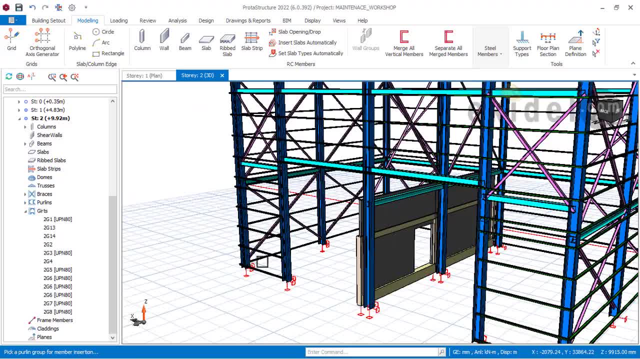 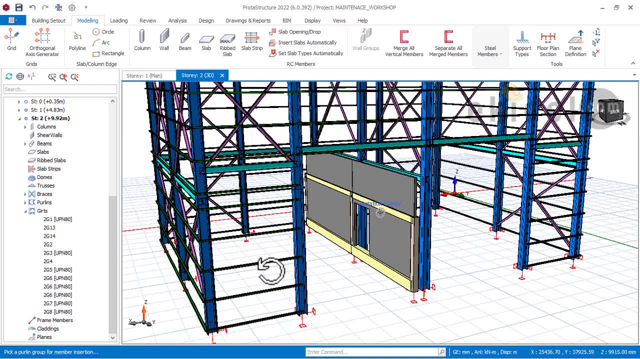 not now but later. Okay, so right now, I'll just go right now Create a cladding on this first area here, because from our model, from our model, it is said that all these, all these pull lines, which is the side pull lines, 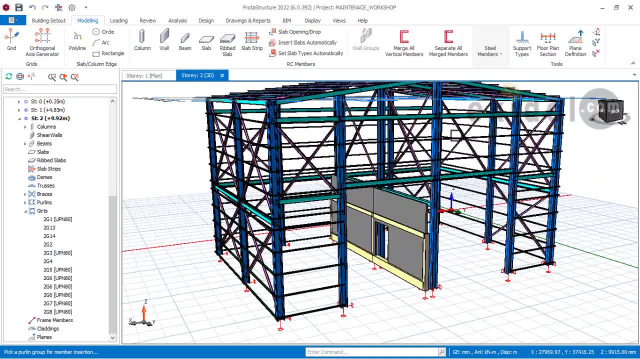 they all have cladding with it. So right now I'll just click on my cladding here, as I did before again, and then come here and click on my pull line, just as you know how to create a cladding before. 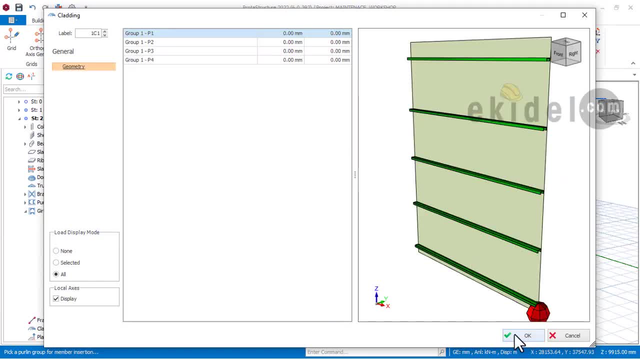 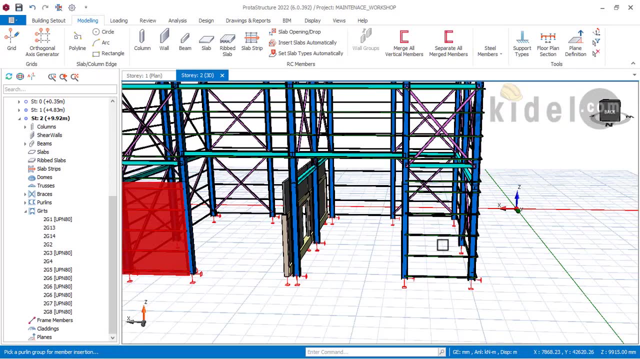 Okay, and then we, once it comes up, I'll just go and say click on, okay, because this one is, it's just a straight cladding that doesn't have an angle yet. So I'll also come here again and then come to this place and click again here. 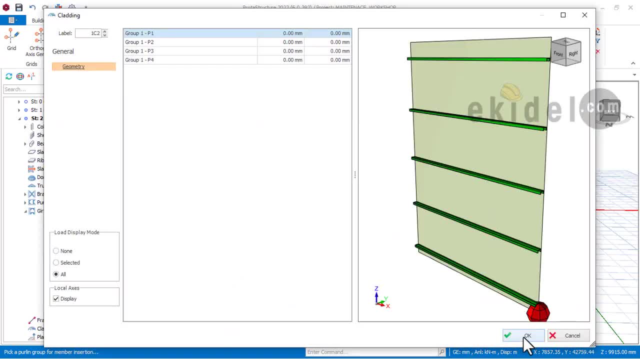 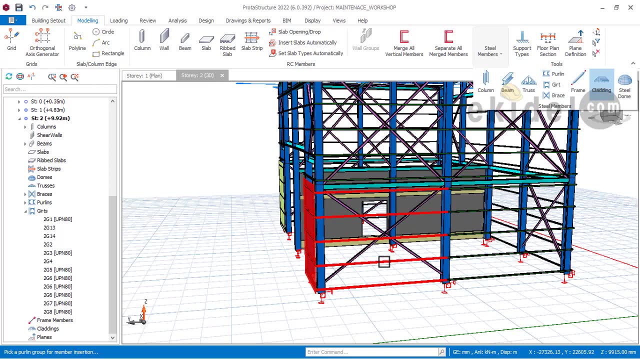 click here Since my, since my cladding is still active, so I can begin to create all my cladding that looks similar. So, okay, as you can see, this cladding here is still active, So I'll just begin to click all my cladding that looks similar. 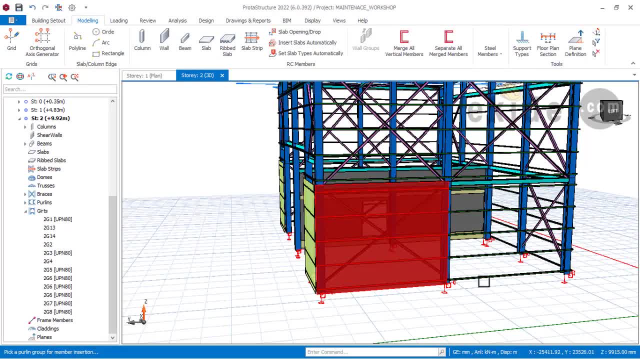 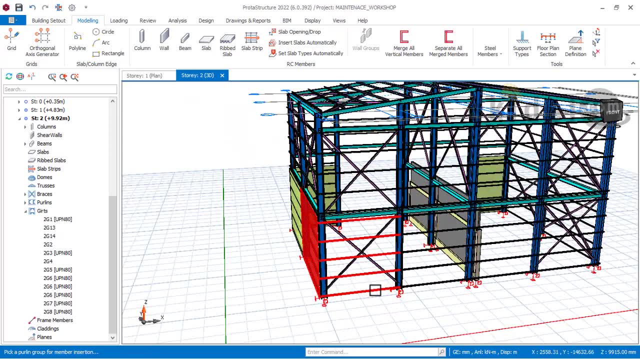 before. I want to enter into the angular cladding area. Okay, so I'll go again right now, then click here and then just say, okay, Now I'll just create typically all the ones that does not require angular cladding Or that does not require level to create your cladding. 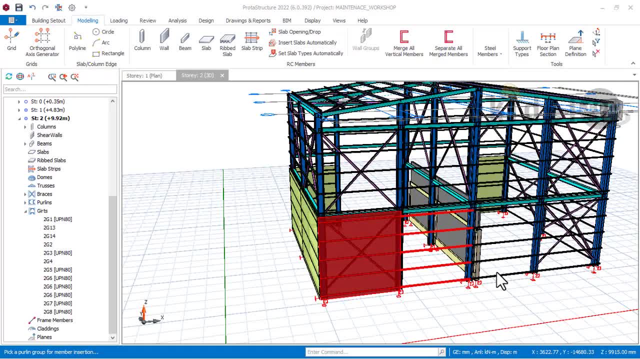 Okay, so I'll just do this right now and then do this again and then continue again here, Do this here, continue, and then come here again, do this here and do this one here. Okay, and then we have created the cladding for that. 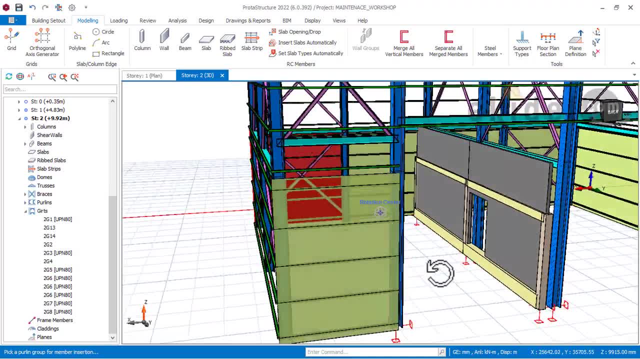 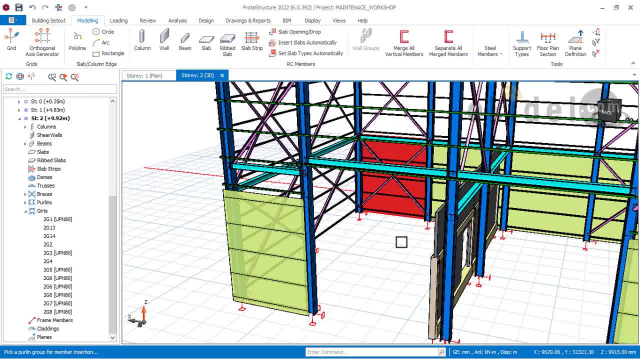 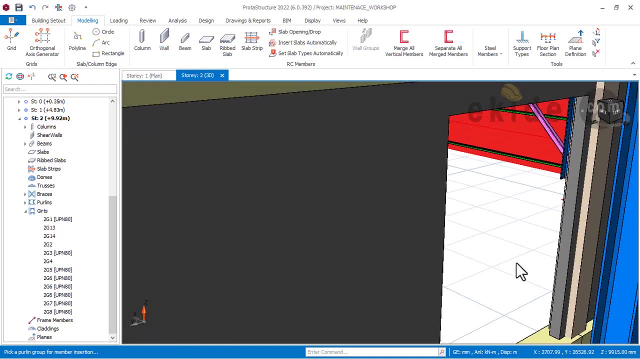 And if you check the inner side of this workshop maintenance workshop building, you can see that there is an entrance door that you can move from this workshop here to this session here using through this door, as you can see it here. Yeah, okay, 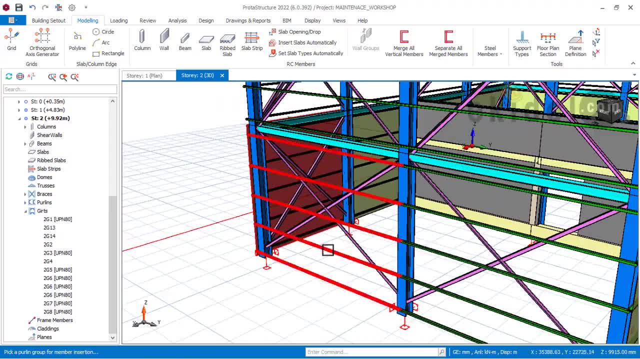 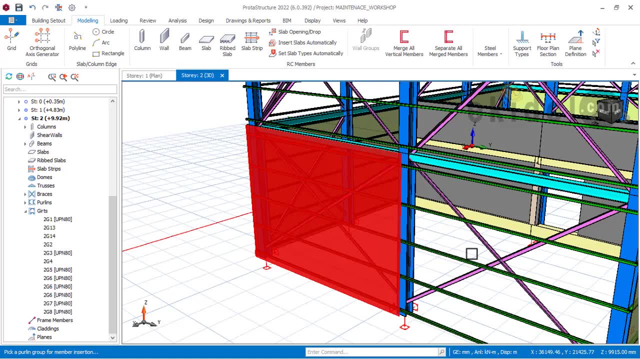 Let's just go back to what we are doing before by creating our claddings Okay, and then click here and then just say okay, and then continue by just doing that right now. So I'll just repeat every or just as I'm doing right now on view. 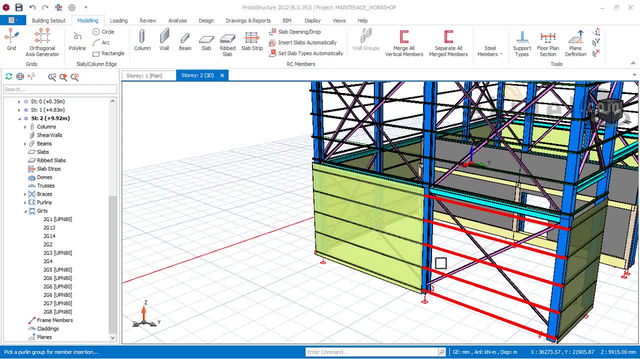 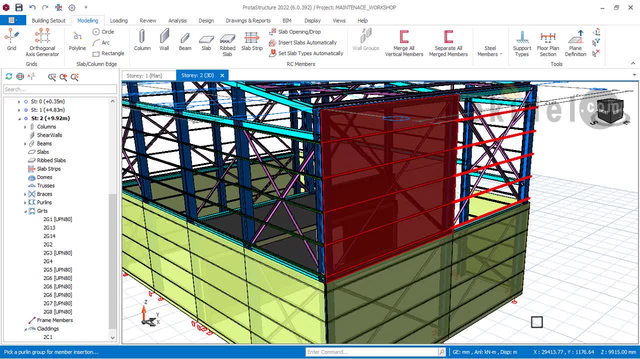 I get to the very stage of our angular cladding: Okay, so I'll do the same thing here and then say, okay here and do the same thing here. and say okay here And do the same thing on this side again. Okay, this other back side. 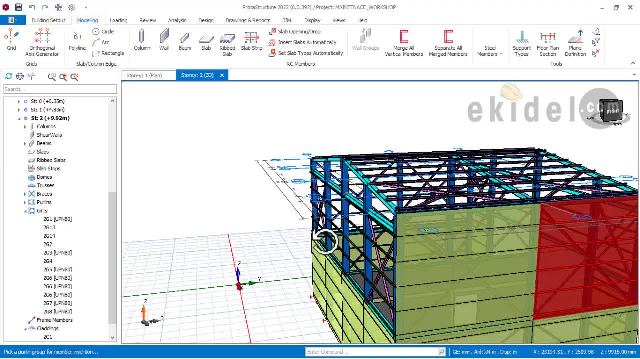 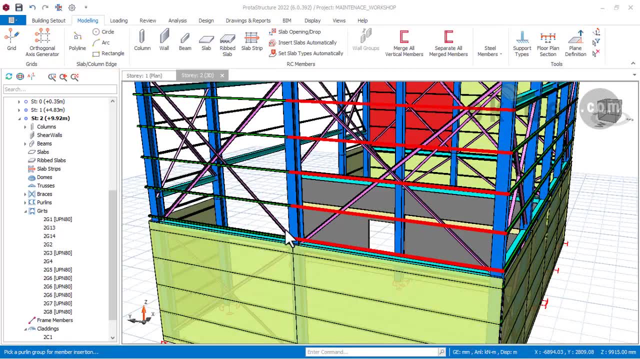 I cannot create a cladding now because it has an angle which I'll teach you just now. So let me just go again and do the same thing for this other side too, And then click here and then say okay, And I'll click here again and then say okay. 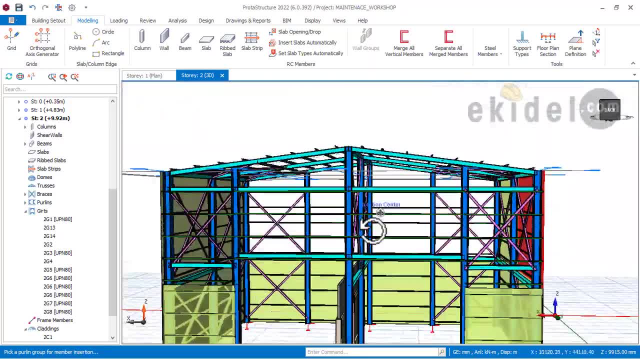 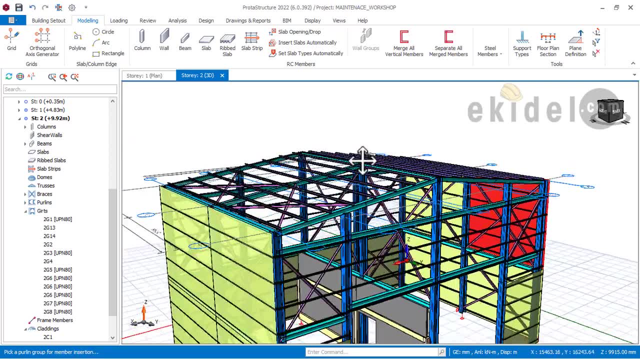 Now you can see that basically I am done creating all my cladding that does not require angle. So these other ones now on this other front side requires angle. So to do that now I'll have to. okay, let me just create this one again. 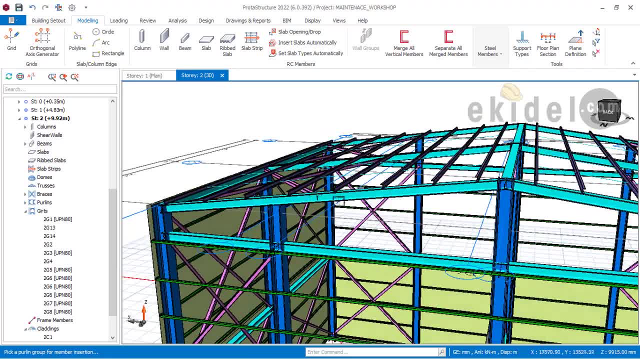 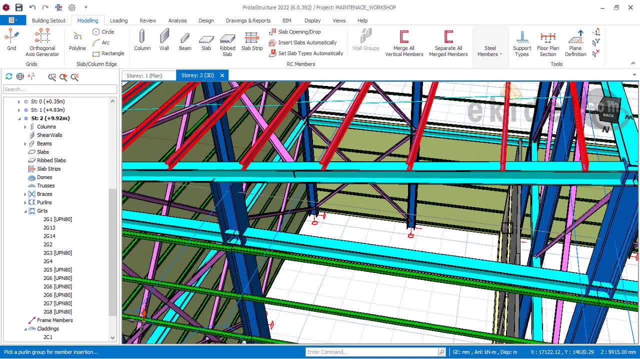 With the cladding for this roof. before I begin to create this cladding that has different levels, I'll have to just create the cladding for this roof now and then click here and then say okay, And then click here and then click again and then say okay. 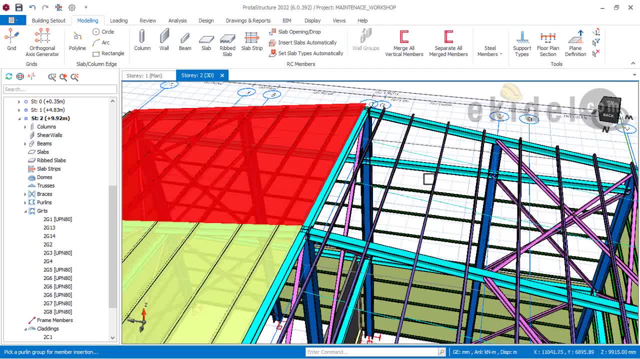 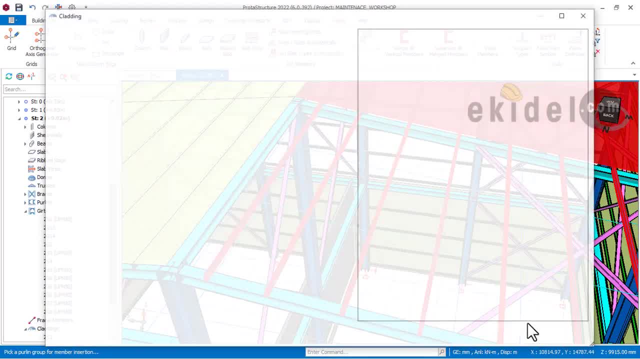 So you have to click on the whole lines and then click again here and then say okay, Okay. and then click here again and then say okay, That's it, That's fine. You can see that we have now created all the cladding. 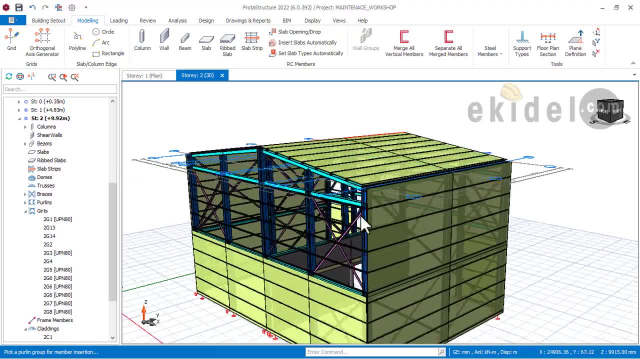 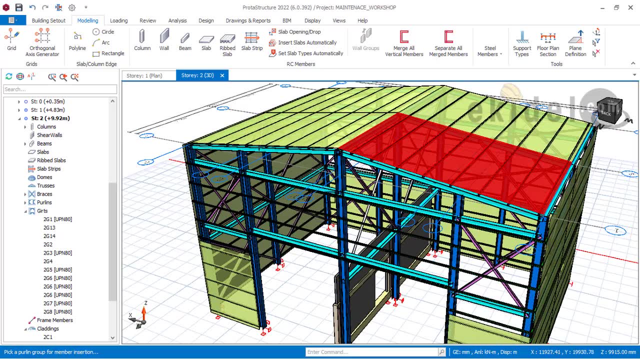 that does not require different level or angle. So these other ones now that are left at this back area and at this front area, now these two requires level for you to perfectly create the cladding that can fit this very shape or this very slope. 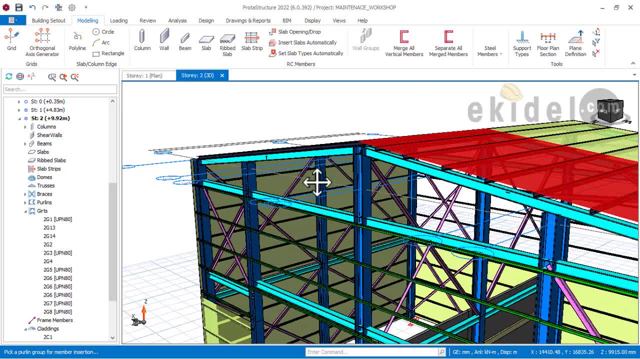 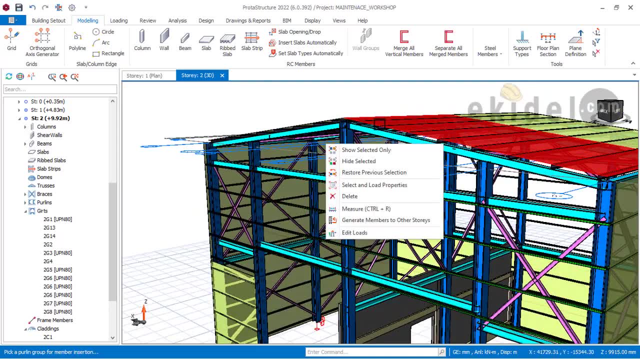 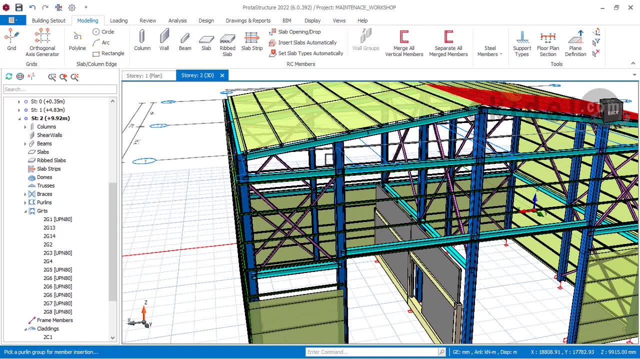 Okay so, right now, let's now begin to create the angle that the sorry. let's not begin to create the cladding that can fit in with this very slope here. Okay so, to create a cladding that have different elevation level in Pintoon 2.0, you have to, first of all, 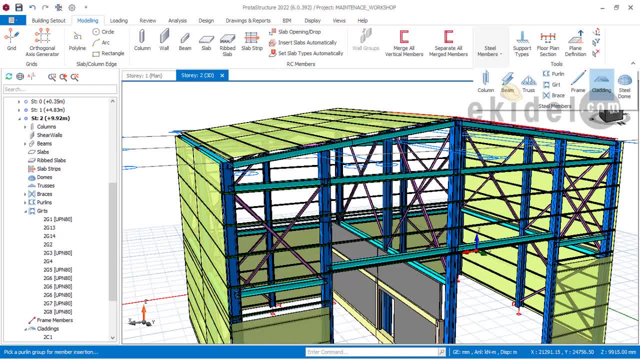 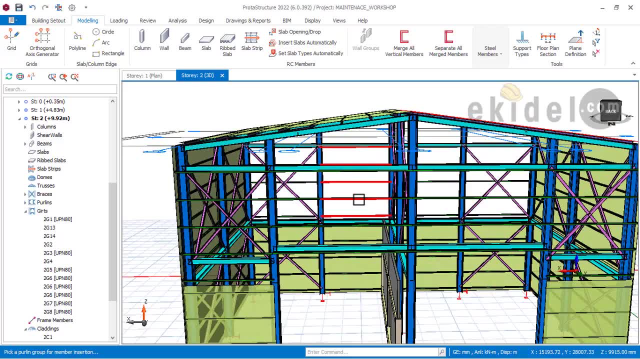 you have to click on cladding and click on the side whole lines. So if I click on this side whole line here now let me say I want to create, or I want to create a cladding that can fit in with this very shape here. 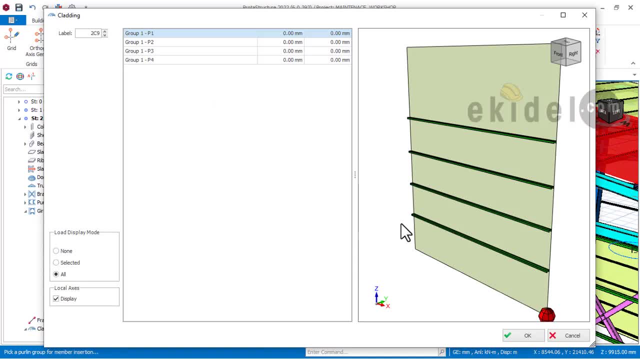 So if I click to create my cladding now, the first thing: if you don't apply the, if you don't apply the sloping elevation on your cladding, or for a steel model that has a slope or different level, this is what you're going to get. 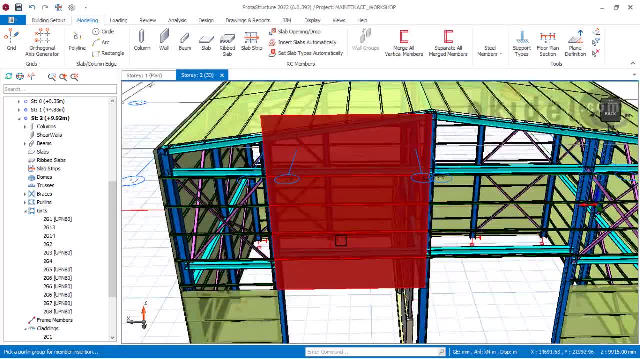 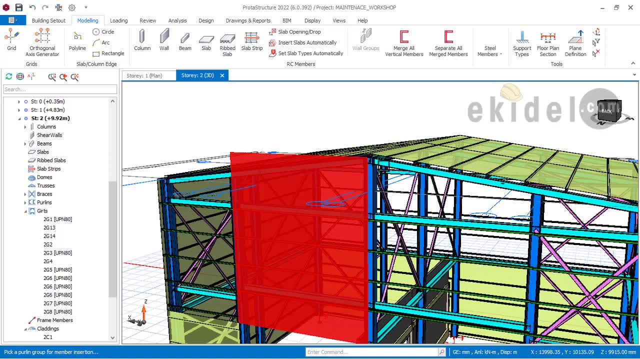 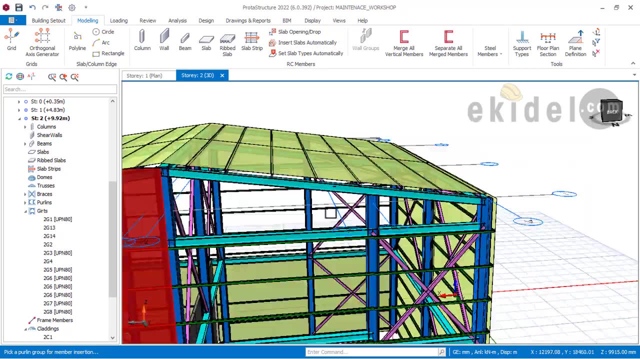 You will see that, basically, you can see that it doesn't fit in to the very shape that we have on display, because basically this cladding was meant to have the same slope, to like flush together with this beam that is falling at this angle. But if you look at what our cladding is now, 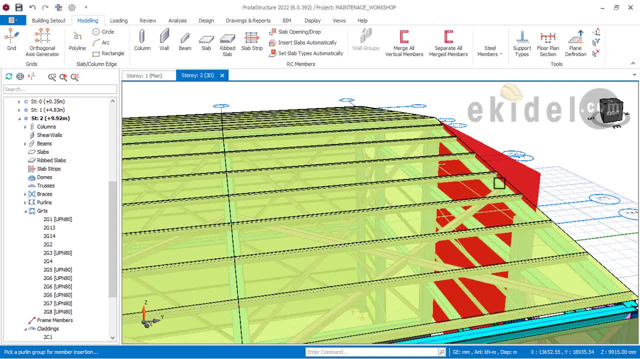 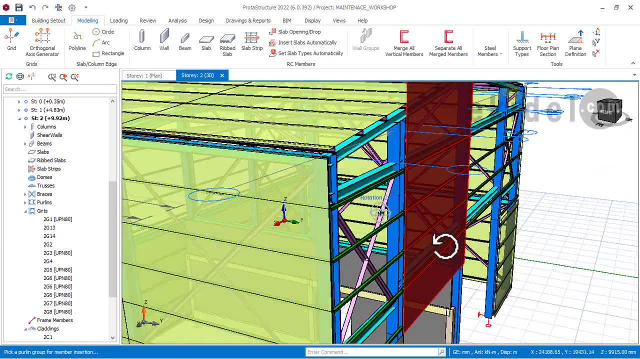 you can see that our cladding is not right because it is not following the same shape. So, basically, this is the reason for this. for this, for this video is to show you how to how to work with elevation when you are creating your cladding. 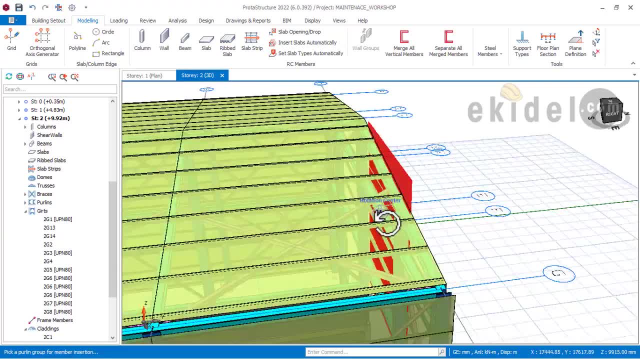 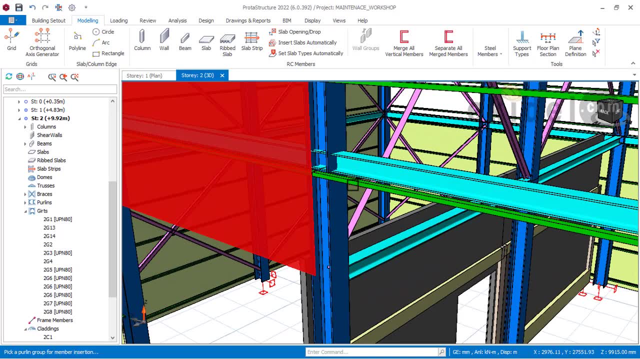 in Pultastro software. Okay, And if you look up also at this end here, you can see that this end, basically this cladding, was meant to stop directly at this at this as this side pull line level, But you can see that it is not extending below and now causing 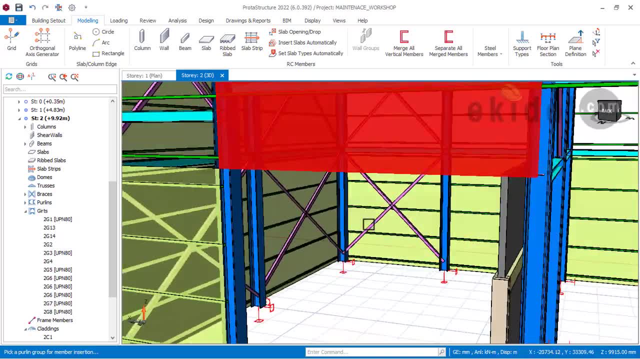 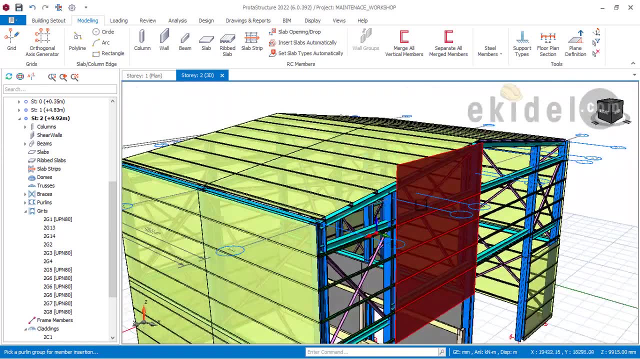 causing an obstruction to the people that are going to enter into this, into this software house. So, right now, so begin to work on that and to then to now begin to correct those things. you have to now begin to do it this way. 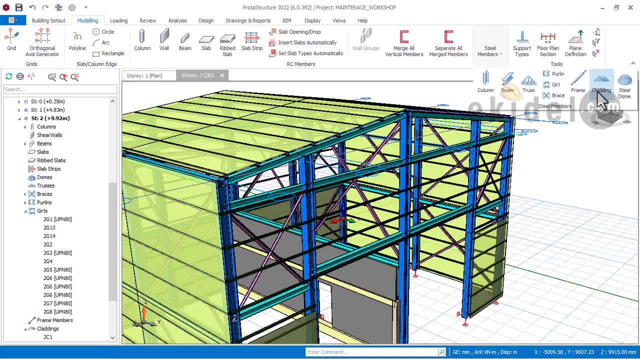 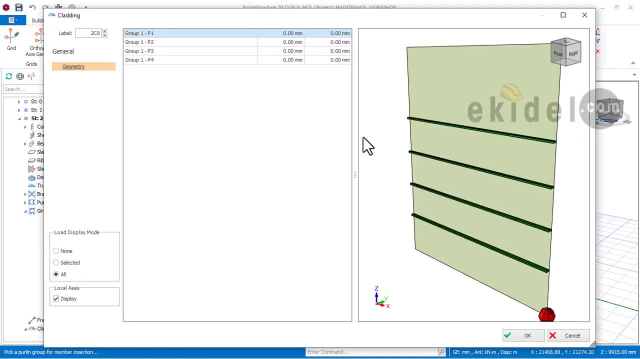 So once you click on your side, on your cladding- okay- and then you click on this place here, once you click on this line of that particular one that has that, um, that shape, the first thing you have to do is to begin to impute your different elevation. 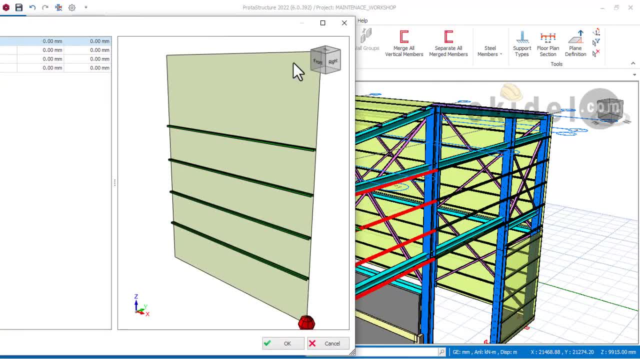 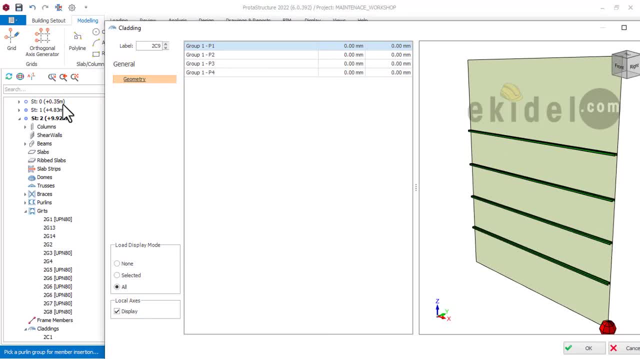 level here Now, based on this structure here, based on this structure here I have already um seen with my height. given you can see that I have different heights. here I have um. I have already calculated those, my 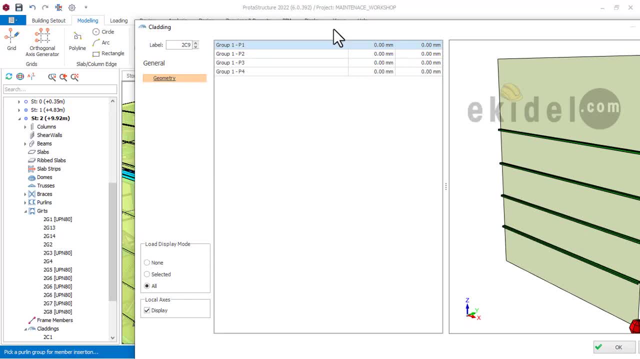 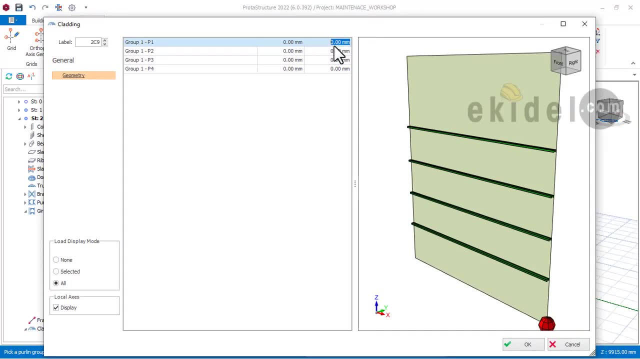 those my elevations, And from those, those, these are the values that I'm going to put to fit in that very shape. So if I go here right now and then put in on this place here, which is the P1,, 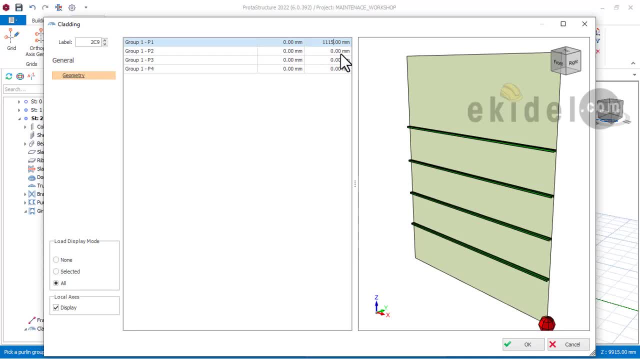 I'll put in 1, 1, um, 1, 5, which will take care of that, which will take care of that excessive cladding that was going um through the, through that entrance area. You can see that I have not shortened this place here. 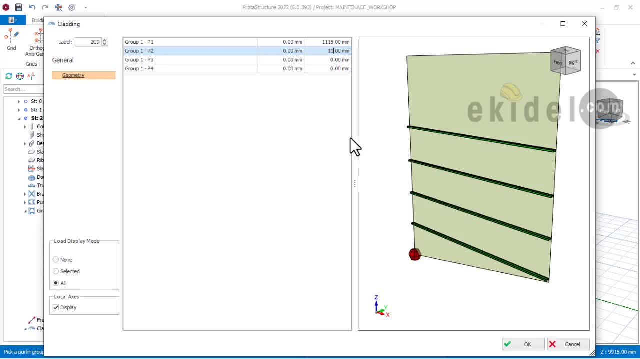 and I'll do again: 1, 1, 5, 1, 1, 5, 1, 1, 0.. 4, 1, 1, 2, 1, 1, 1,. 2, 2, 3, 4, 1, 1, 1, 2, 0.. 6, 5, 6, 5, 8, 1, 1, 1,. 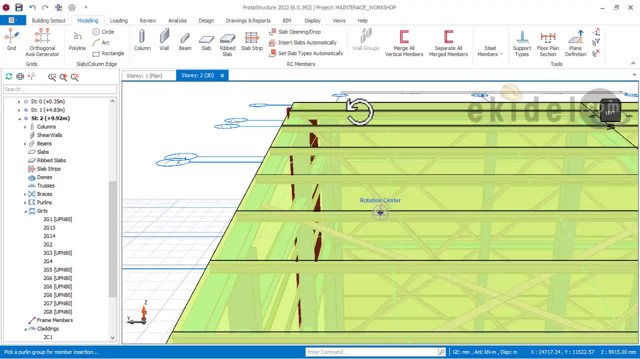 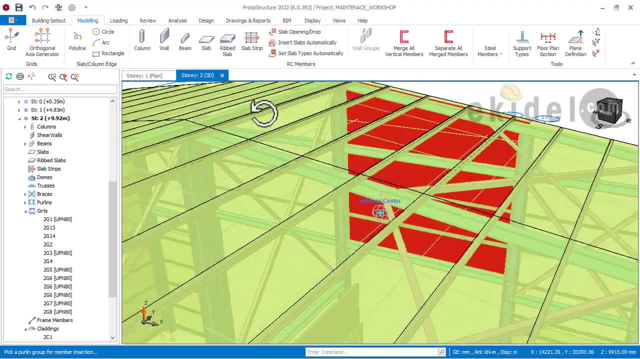 5, now a perfect slope that flows directly what i want to consider right now. if i've used one for this point, you can see that they are. they are being sloped based on the side, based on the beam beam sloping, as you can see that, and also on this entrance side. you can see that. that this cladding, 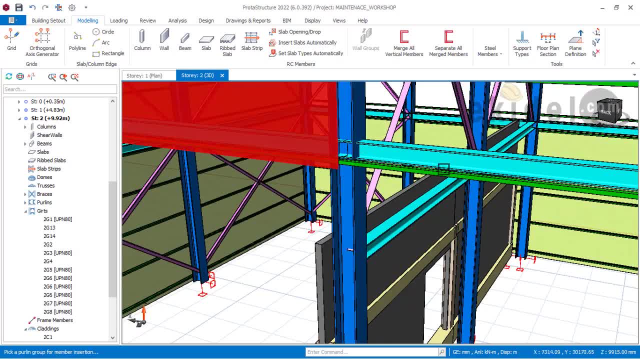 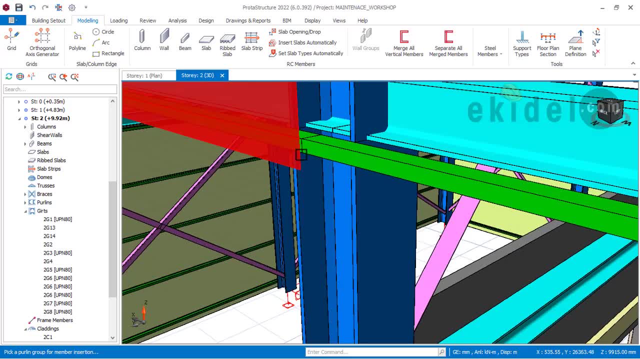 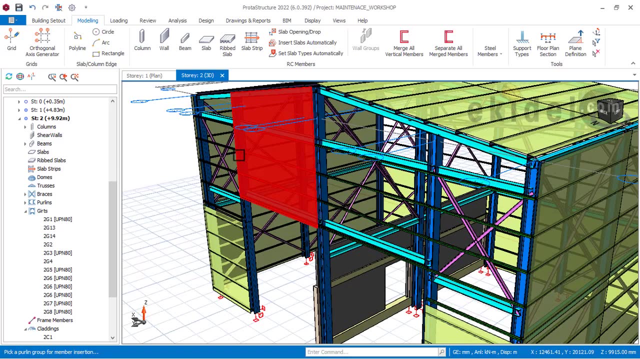 now stops directly at. at that, this cladding now stops directly at this side pole line, just giving you just given a little allowance of at least 50. you can see that now. you can see that if you didn't put this, um, if you, if you don't have to put that, that elevation, this is what you're going to get. 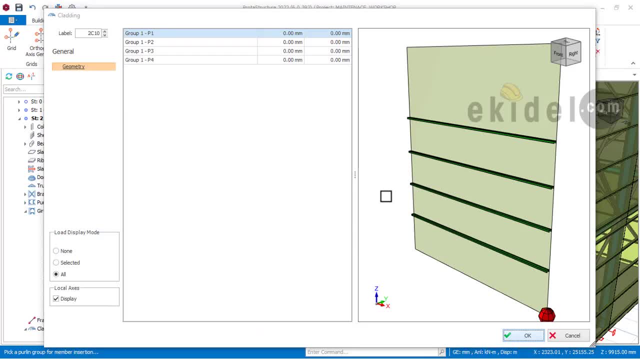 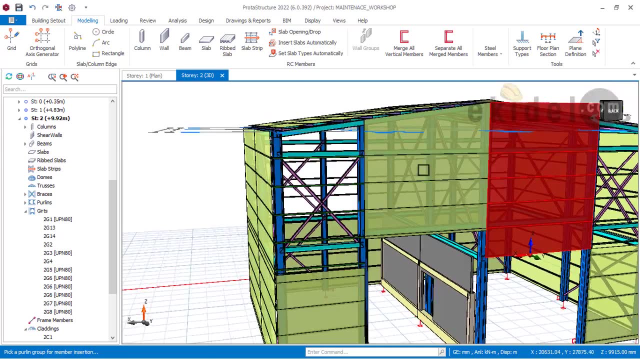 you'll get something like this. let me just put it on this other side now. you will get something like this: you can see how that this one here that doesn't have different level is not the same with what we have here. this one that that doesn't have level is not being shaped based on this. 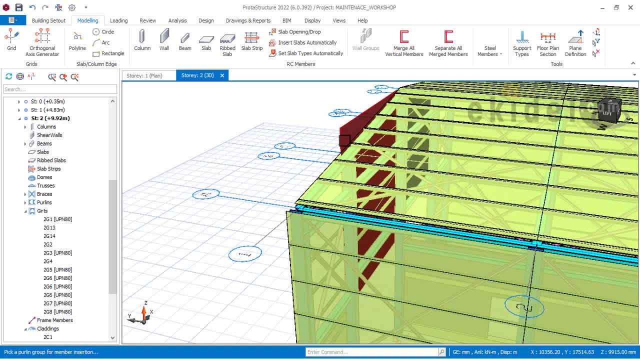 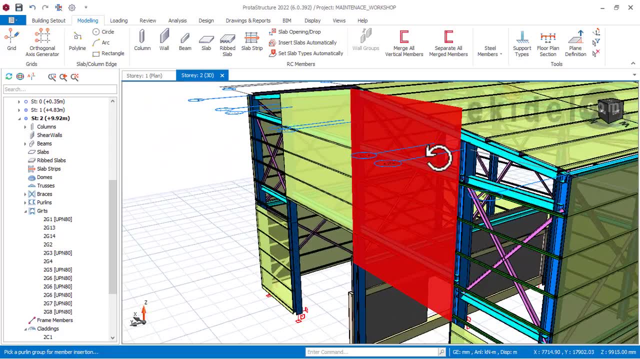 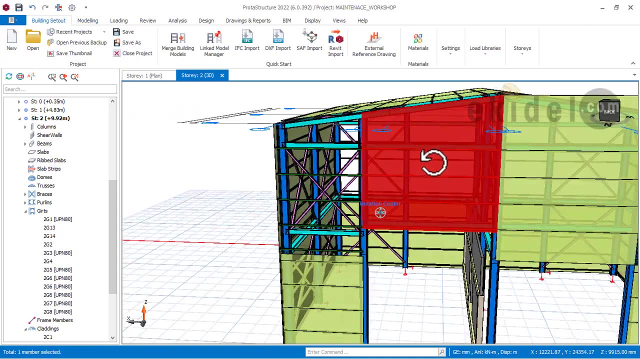 particular place. now you, you can see, can't i trim it? there is no trimming of cladding. on photos of twin pins, too, you cannot trim cladding. the only thing you have to do is to work on the elevations. okay, so you can see that this other one here, this other one here, is perfectly placed because we used angle. 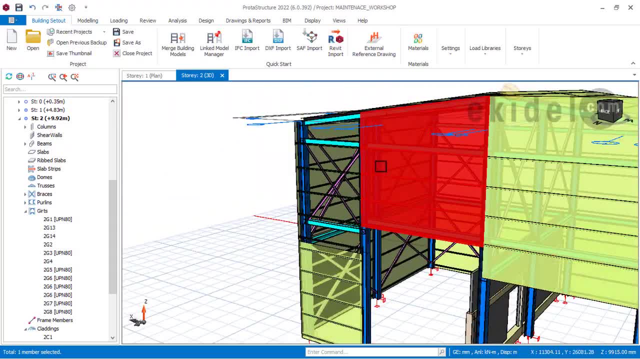 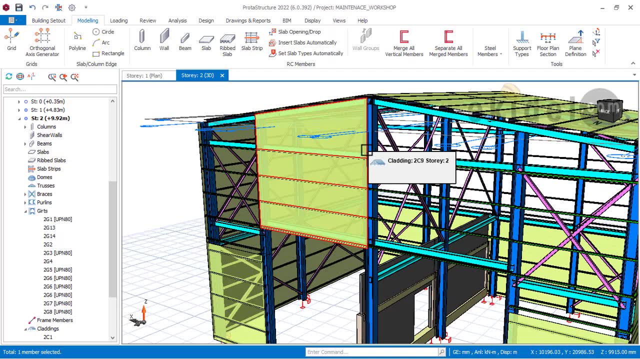 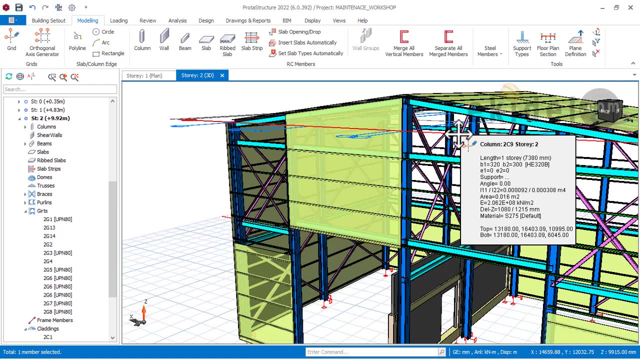 and you can see that it has been uh it, it is also flushing with this, so i'll just remove this right now and then use the other angle. now, whenever you are working with angle, know that there is what they call um anti-clockwise and also clockwise, so this one that we did now is called a clockwise um cladding. 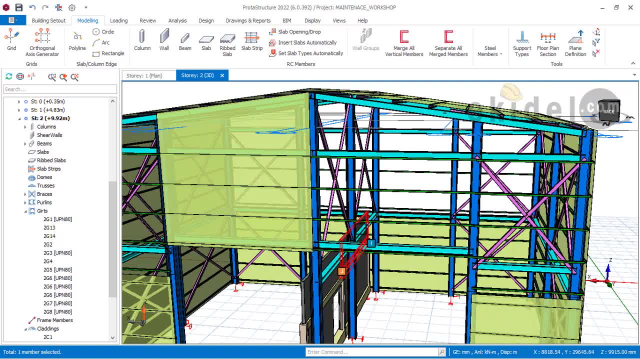 and this other one here that i'm going to put on this side now will be the anti-clockwise, which is just the reverse. okay, so right now, i'll go again right now and then click on what cladding here, cladding here, and then click on what here and then click on this place here that says, uh, click on the. 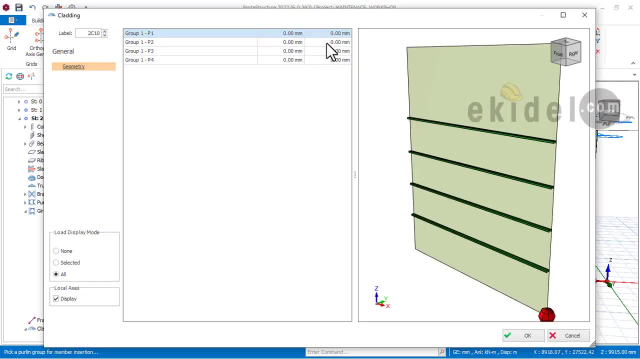 cladding here, sorry, on this um line, here and now. i'll have to put in my value here the same thing: 1115, sorry, five, again one, five, and then here one one, one, five now on this other side. now don't forget that we put that: uh minus six, five, um, six, five, six on this, on this, before now. we are going to put it now on. 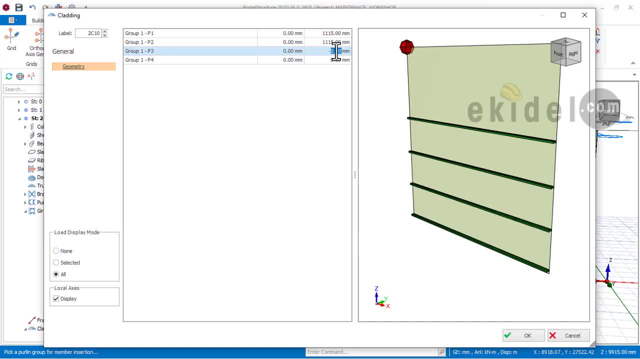 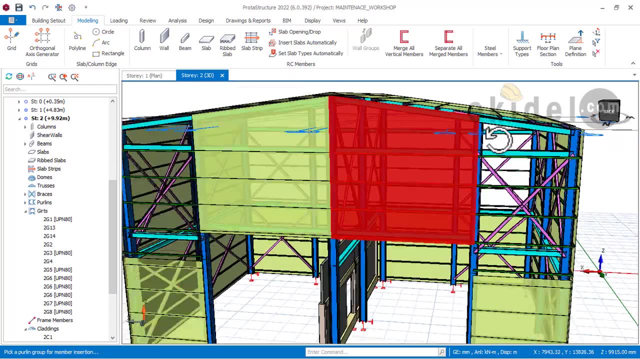 this p1, on this p3, sorry minus six, um, six, five, six, and i'll come here right now and then click on what. okay, so you can see that it will just slope in now, as it is okay, as you can see that, so right now, we have now successfully created this other one here now. let us now create for this. 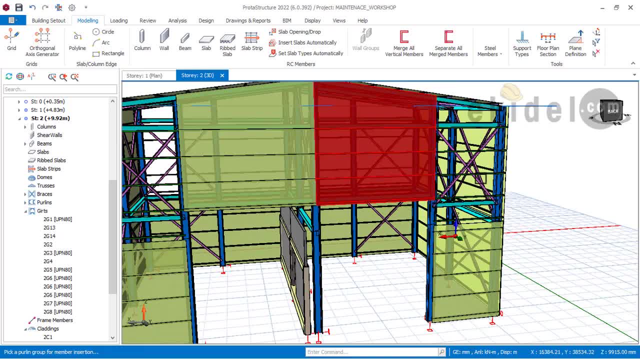 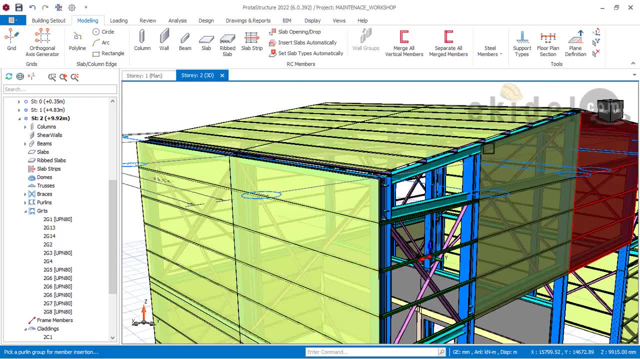 other, um smaller one here also, because what we did was for these two here now. let's now also create a cladding for this other side here, which is also having that kind of sloping issue. so we also click on that, on the on the cladding. first it is the active and then click on this other one here. 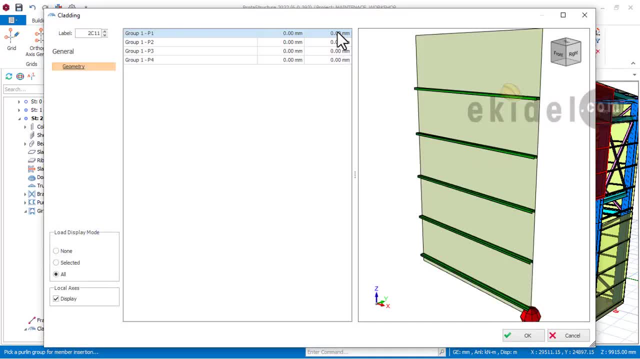 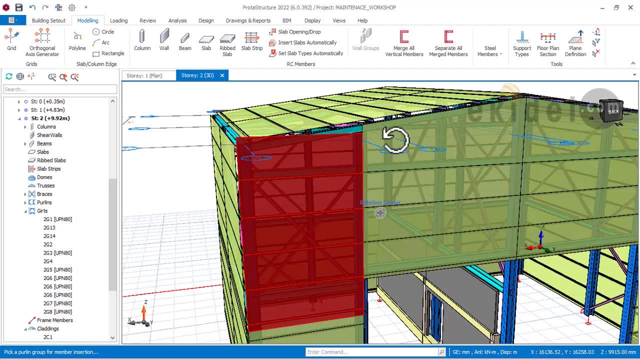 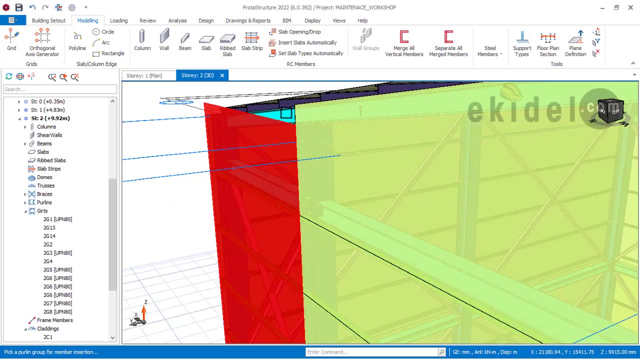 okay, now, once i click that right now, if i do not want to put this um this, this um elevation, you can see that it will not also fit in, so that's why you must. you can see that it is not fitting in um, it is not um trying to it like. it is not corresponding to what we have, as you can see that. 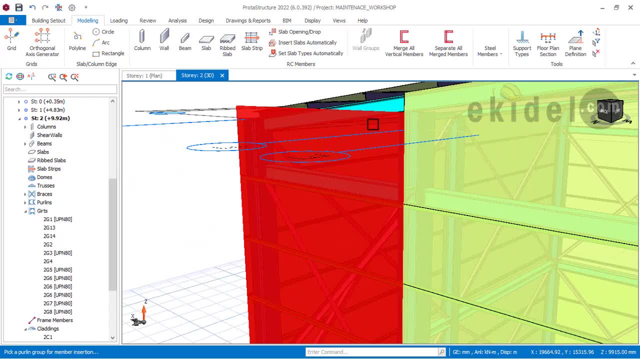 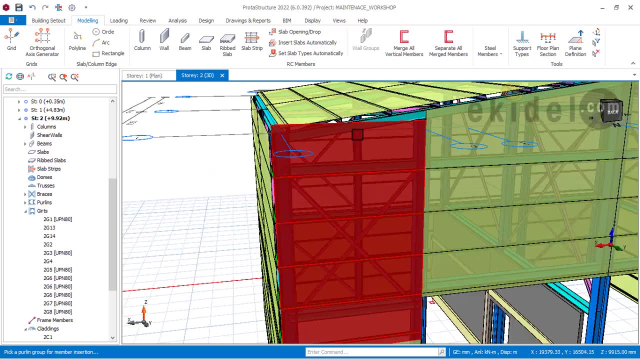 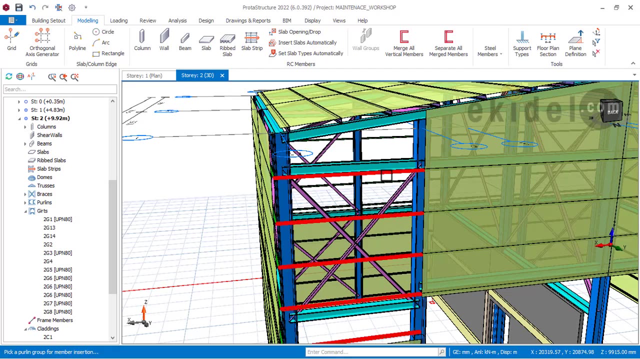 it is not having the same shape, so that you must work with elevation when you are working with either um steel structure that have different um, like different slopes. okay, so to be able to do that right now, i'll just have to delete that just now. i'll remove that and then put in a new one, and 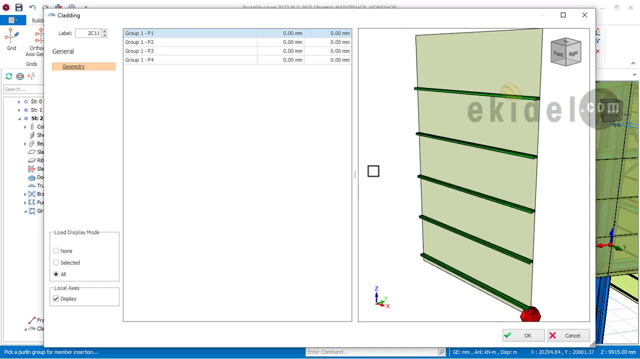 they click on this. now why i'm putting that right now. i'll have to work with the elevations. now. this right now have different elevations because it's because it is on a different um area entirely, so i'll have to work with the elevations here in this one. now we have to put in p one to be zero p. 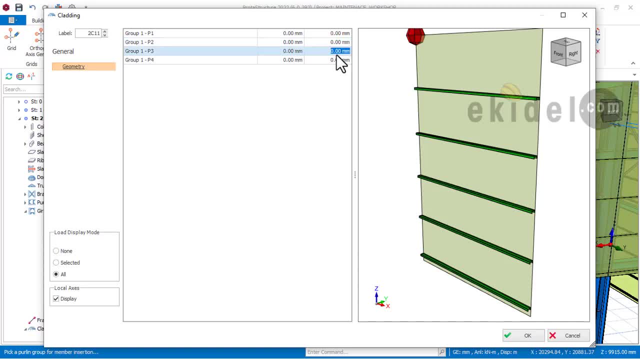 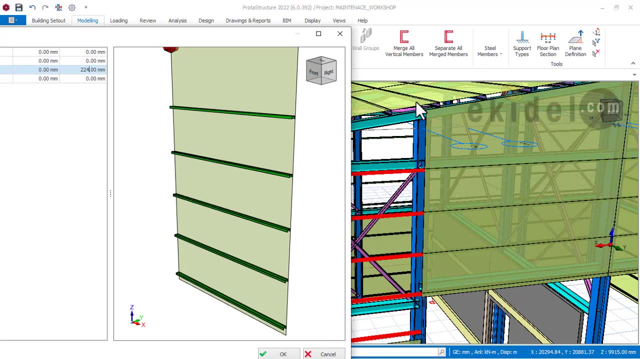 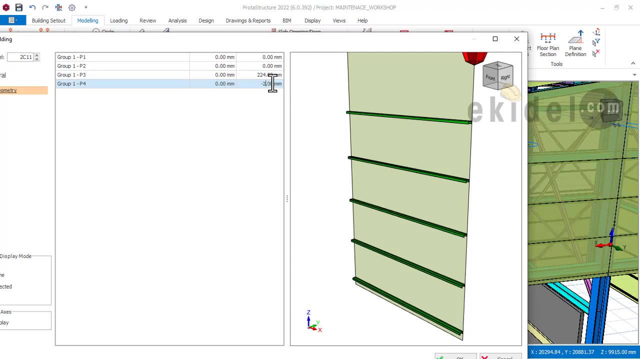 to be zero. and then we come here right now and then put in p3 to be two to four to be able to slope um together with this level here. so this level for my own calculation for this warehouse building is two to four and for this other side now is a minus um 200. 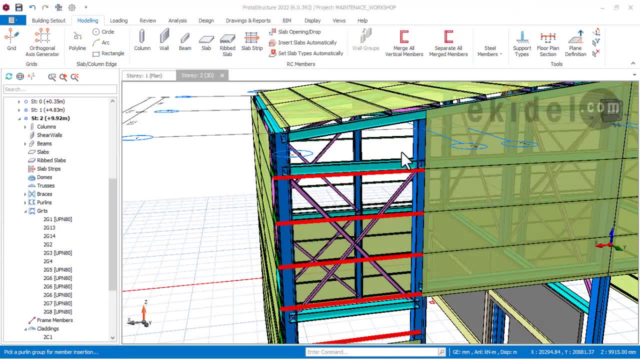 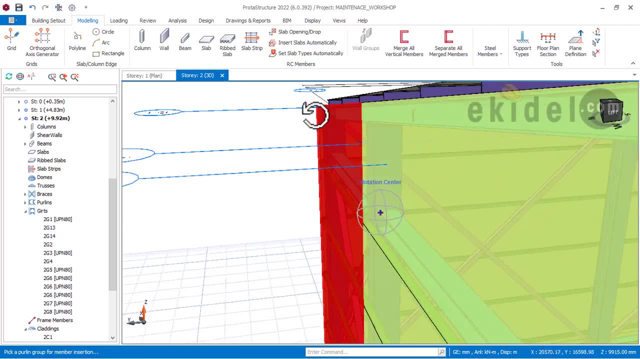 if i do this right now, then just say, um, okay, now you can see that it will just flush directly as it is, as consider. so you can see that it has flushed directly, you can see how they are being flush, as you can see that they have been flushed. and if you also check on this other side too, you 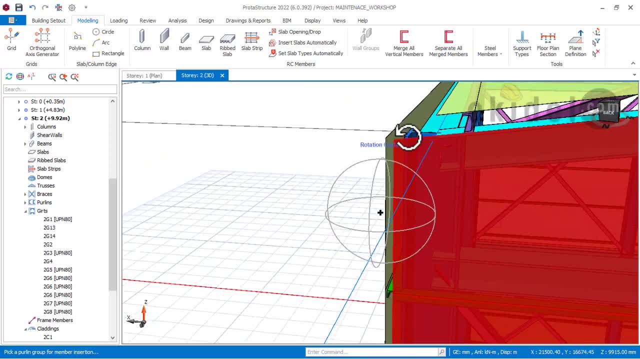 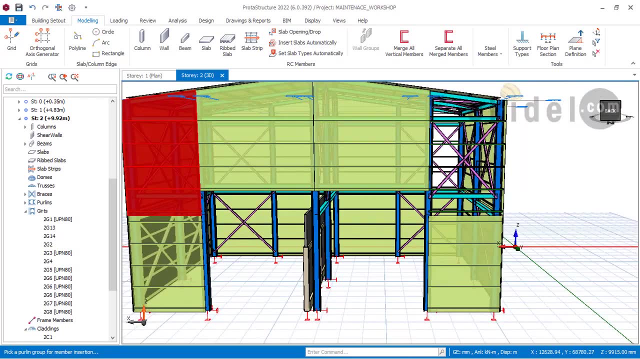 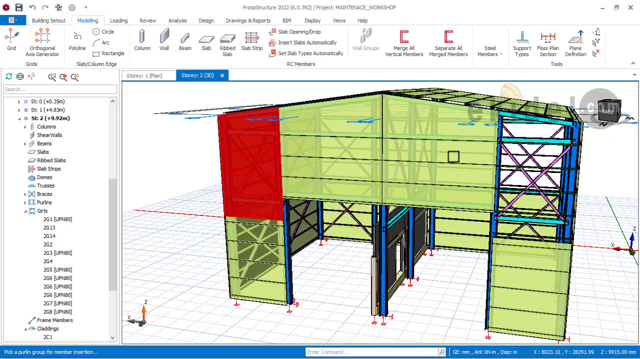 can also see that they are also perfectly um placed, as you can see that they are flushing with this now um, how to get your level basically on um on a steel warehouse, reading is very, very difficult. That is why we have what they call Ekidel Mentorship Class. 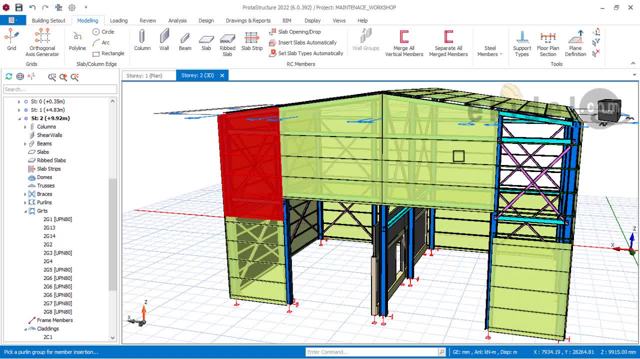 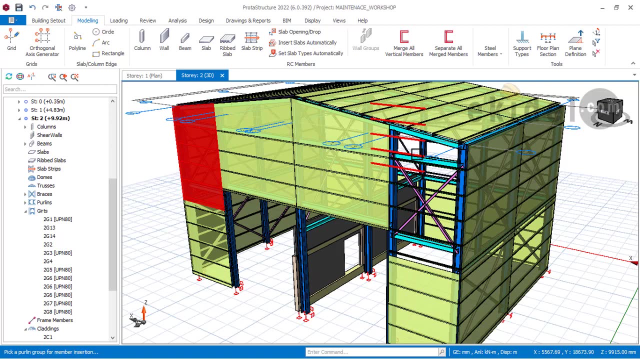 It is not free, but the reason for that class- which is a separate training where we use Teams or Google Meetings to share our screen while we are training you- is to make sure that you get conversant with this software and also how to design either street structures. 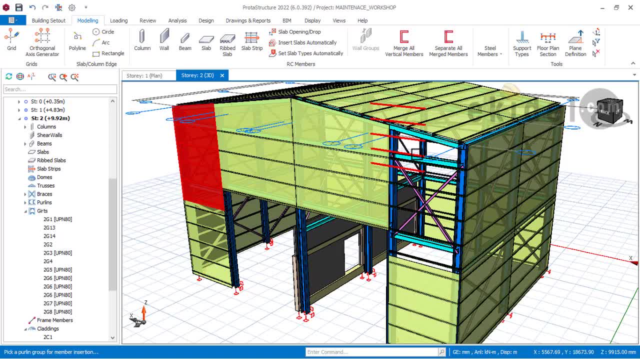 or what they call concrete structures. Now we have a lot of syllables that we will train you so that by the end of that training you will be able to know everything that is on the syllable. We have also included the link down below. 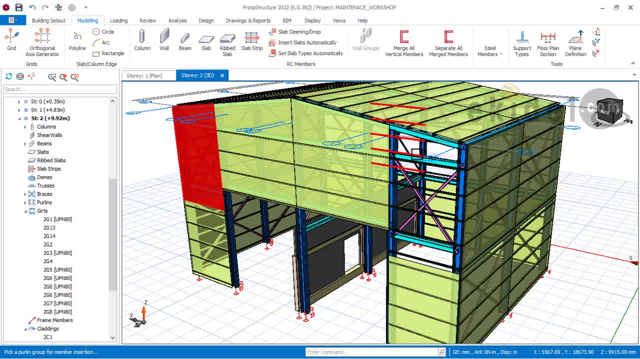 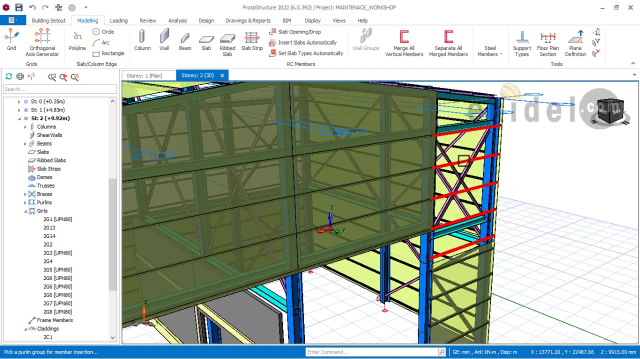 So if you want to know more about the syllable, you can check the link down below and know about our training. and it is not expensive and also it is not that low. So let's now create again for this other option So you can enroll for your own specialization. 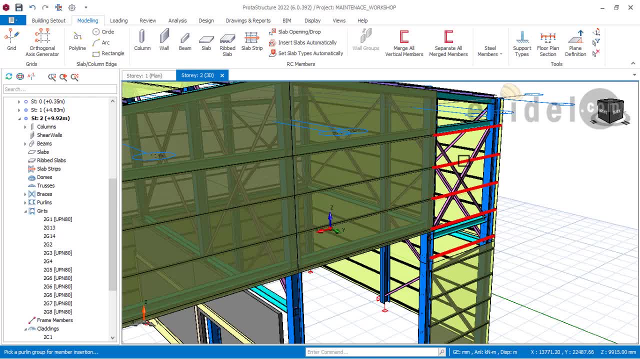 I have child training on social design, which will train you on steel design and also concrete design. And to know what you're going to achieve by the end of that training, just check on the link down below and go to our Ekidel Mentorship class. 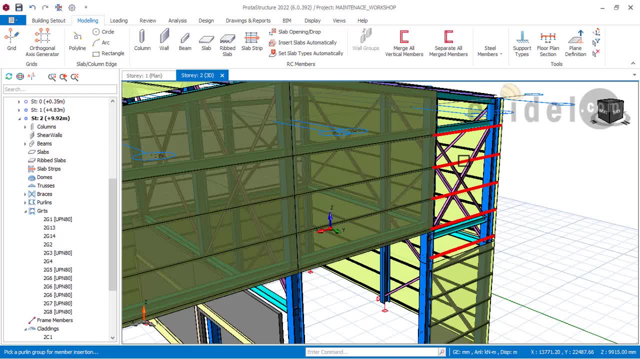 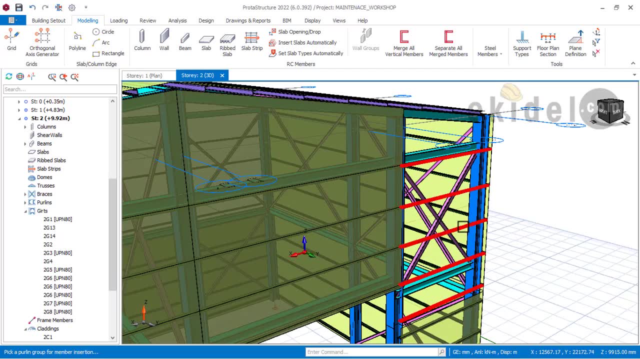 As you can see it here, and also, by the end of the training, we are going to give you a certificate for that. So let me now create again for this other side here Now. create again right now and click on this place here Now, knowing that I said that: planning when you're working with a particular subject. 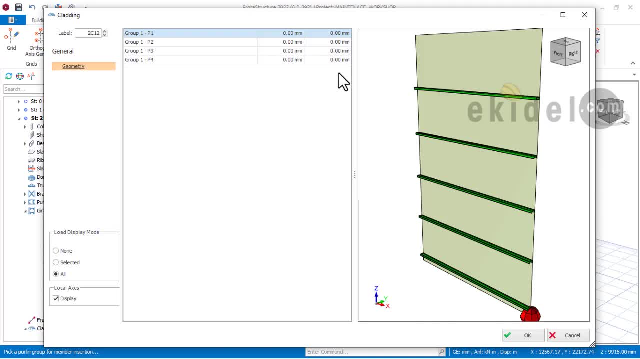 you need to create a certificate for that. with slope, you have to work anti-clockwise and clockwise. so the data we did before was a clockwise one. now this other side. now i'll still make this place to be zero and this to be zero. now. p3: now, instead of having p3 to be two to four on this case, now i'll have to make p3 to be. 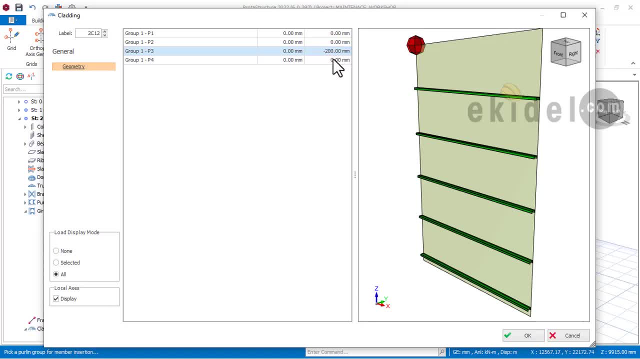 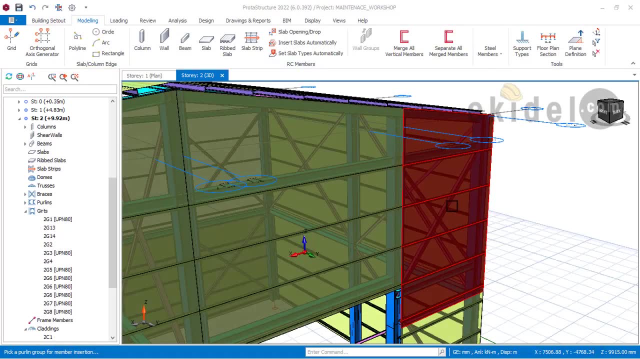 minus 200 and then p4 will not become two to four. so that's how it it it works. okay, i'll not come here right now and then click on what okay here and then you will see that it will just fit into what we have here, as you can see that. so you cannot see how we have created a 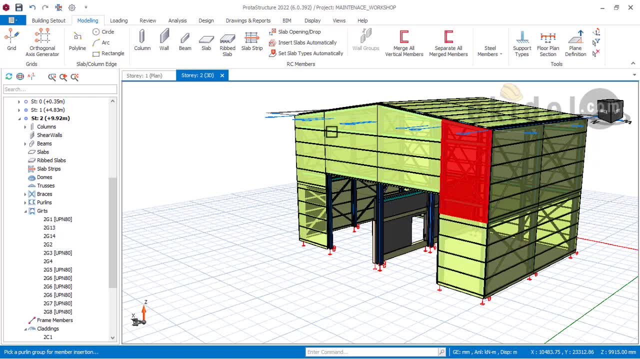 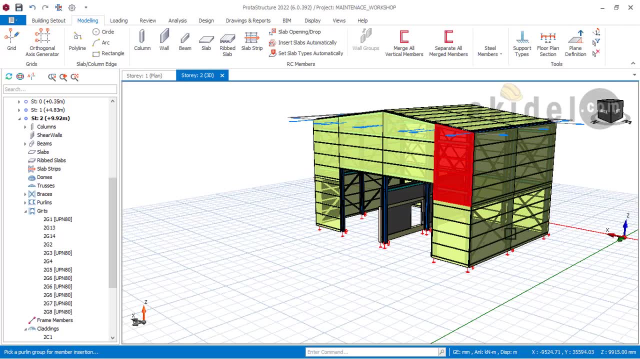 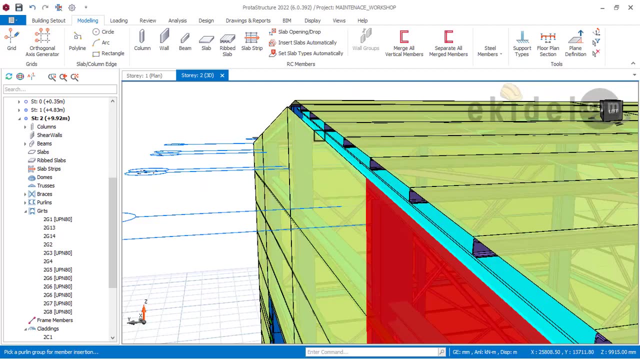 cladding for this um, for this upper um, for this upper level here, is different from how we created level for this lower one. the reason is because this upper one here requires a slope to work with, and then you must work with the slope while you are putting in your own cladding, and which is 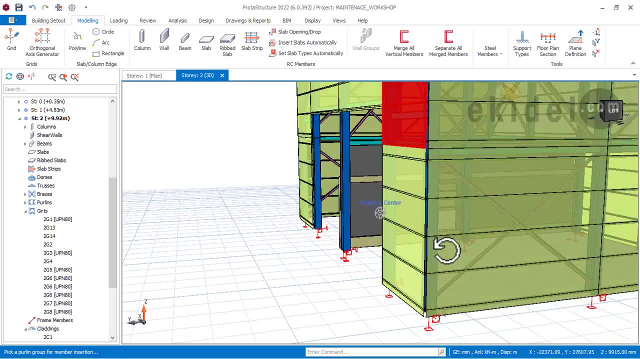 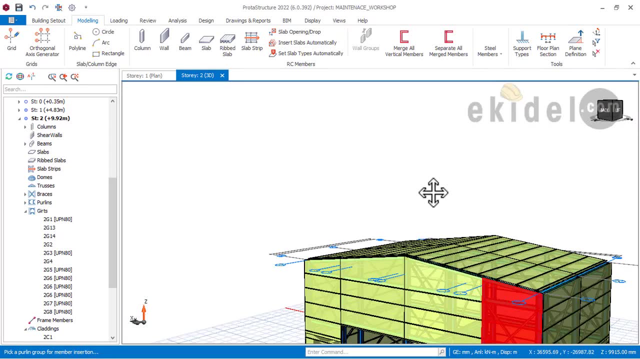 different from what we were doing before here, because this other one here is just a simple way of putting cladding that does not require any kind of different level or slope. but this other one, this other side here, requires you to work with that level, okay, with that level, before you can fit in your cladding. 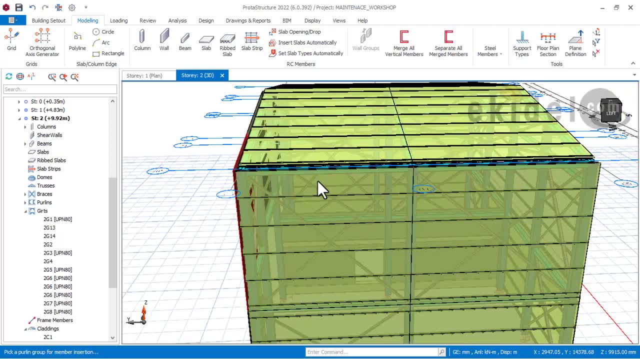 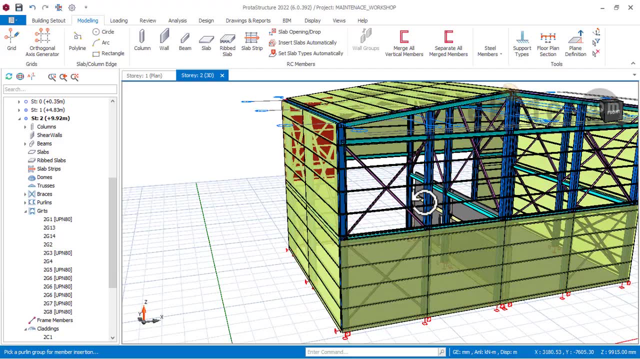 based on the shape of your steel structure model. okay, then, let's now walk on again to this. back here. so if maybe you didn't grab what what you did there, put attention here for also to grab what you're going to do right now. okay, so to put a cladding here on this. back now. 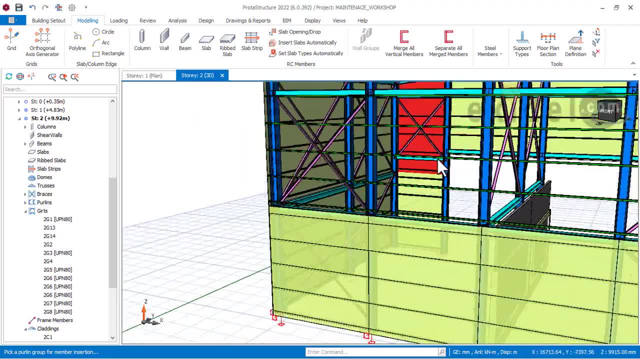 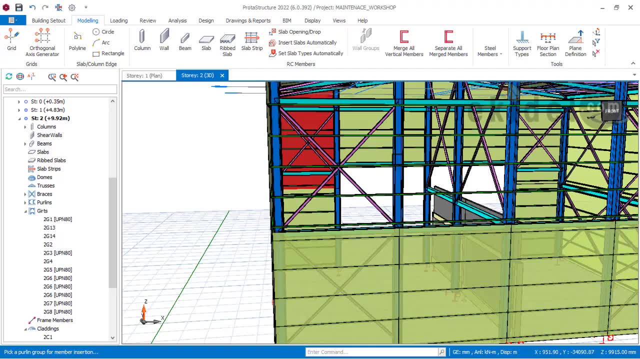 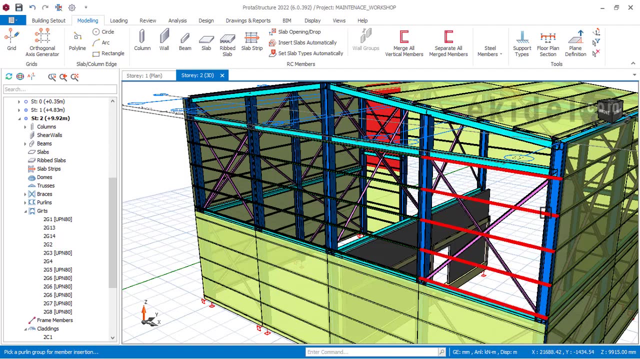 for this back side here. right now, let's let me start. i can see that this back now it's been divided into four partitions, as you can see that from this column here to this column here is one partition, and from this to this is 2 partition, and then from this to this is 3 partition and then from this to 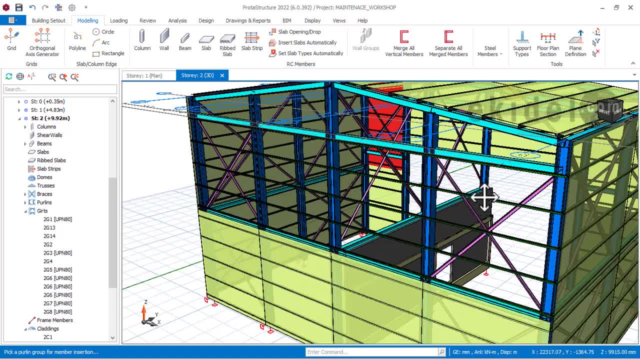 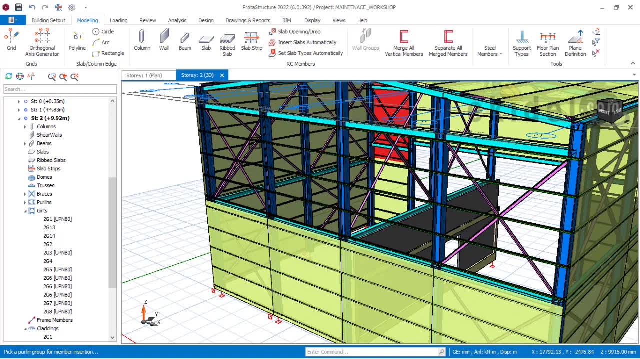 this is 4.. so as it's been divided, so also are the discard lines divided, and since the combat lines also, we have strains one, we have two, and we have three and we have four, and since the demonstration lines are divided too, so so also we are also going to divide, as 잠깐. 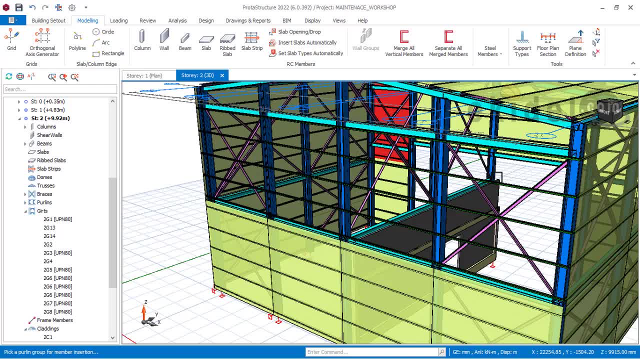 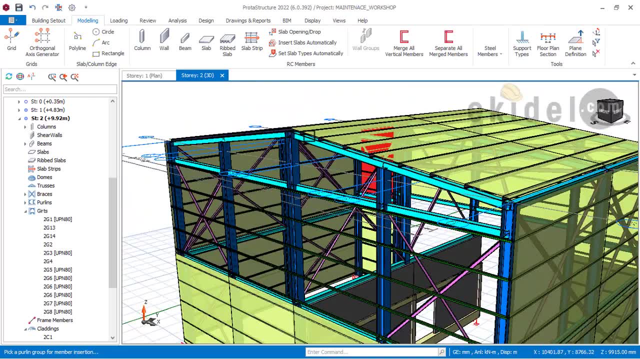 going to place our cladding based on how the pull lines are being divided, and don't forget that this also have a slope. as you can see, it has a slope at the backside here, so we are also going to work with this slope and make sure that. 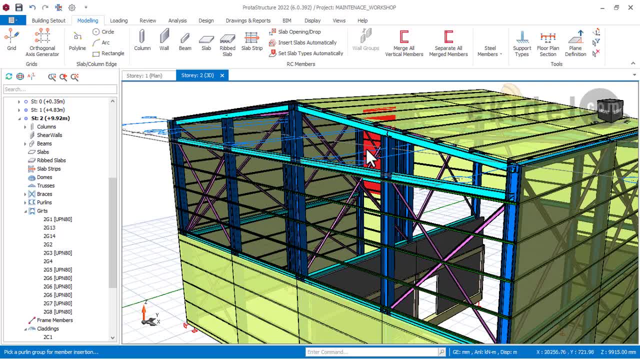 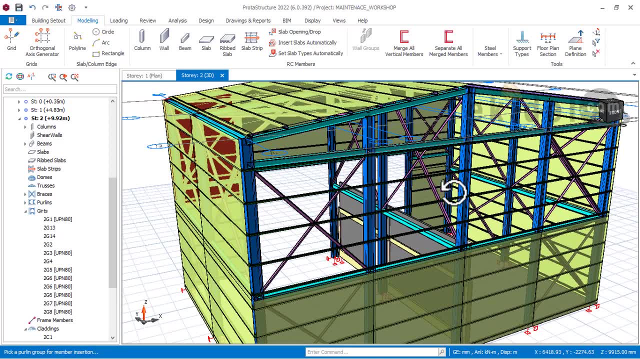 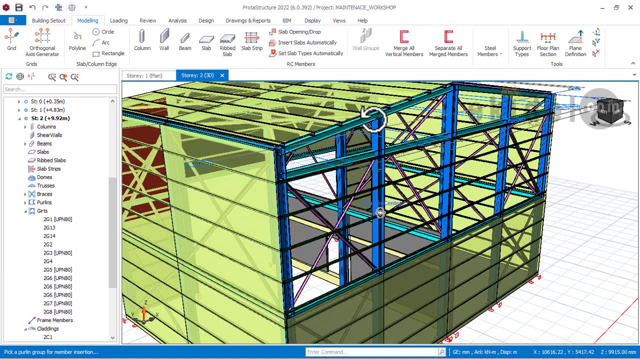 our claddings are going to fit in based on the slope elevation level. okay, so right now, let's not begin to now create our cladding based on this first idea. now, most of you guys- might most of your- your software might be lagging when you're working with product structure. but you can see, right now mine is not lagging. 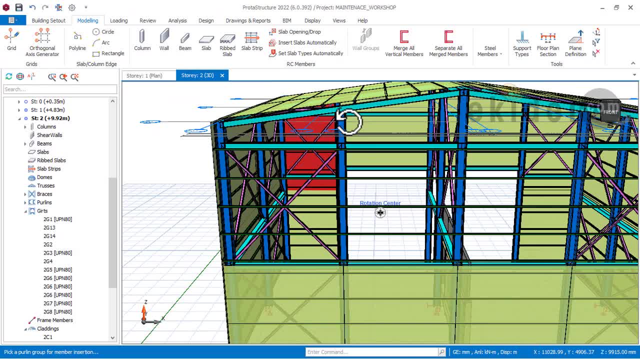 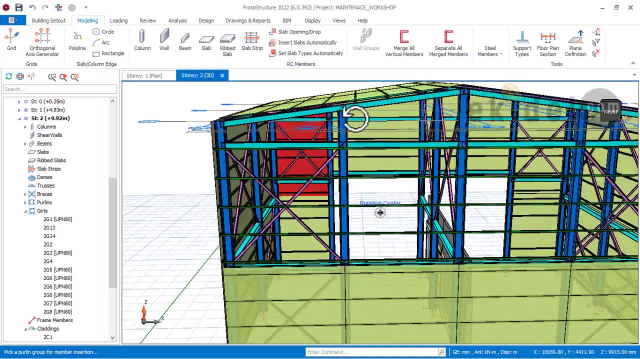 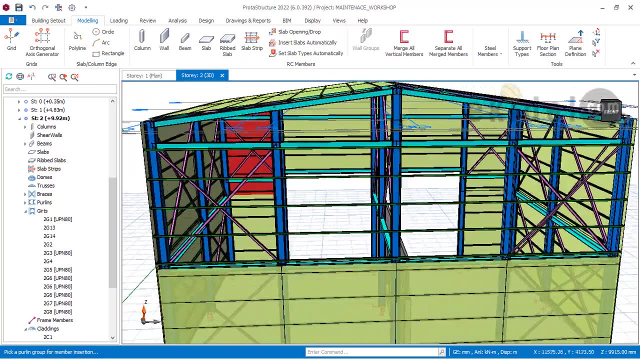 this lagging principle or lagging, doesn't really depend on the capacity of your system. so even if you have a low RAM system or the low speed system, you, you can still make your product structure to be very, very fast. and there is something you are, you are you, you are going to purge into. 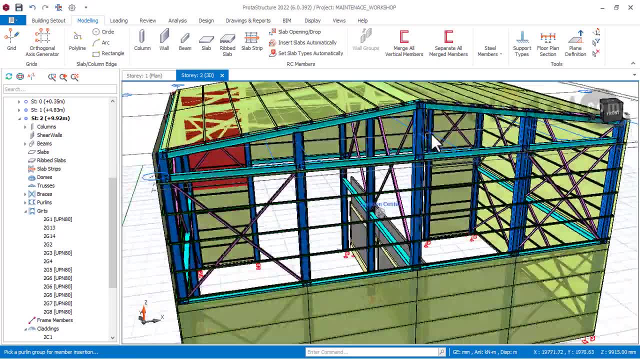 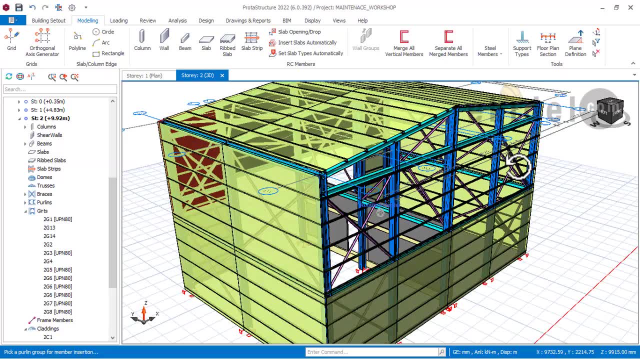 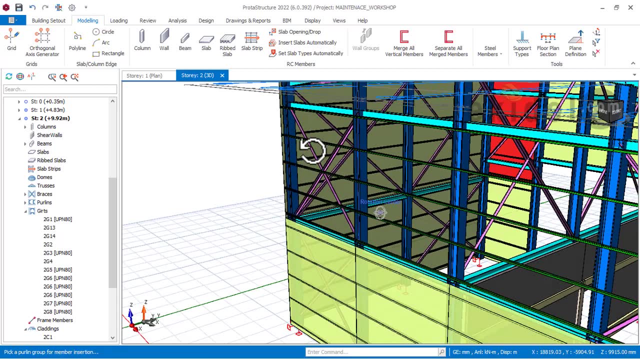 your software before you can begin your modeling, else you will spend so much time while you are modeling and can see that you can be able to make your 3d view very, very fast. okay, but that would be a different class for a different day. so right now, I will now begin to create my own cladding here, and I'll start with. 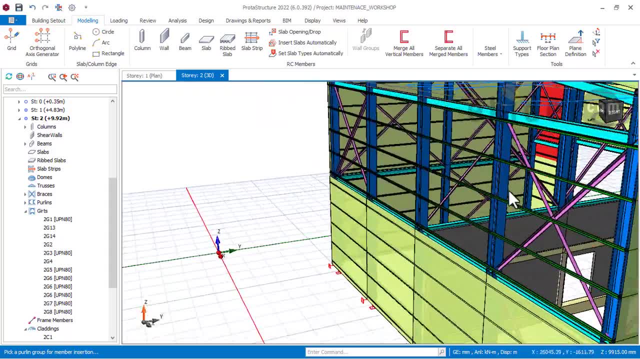 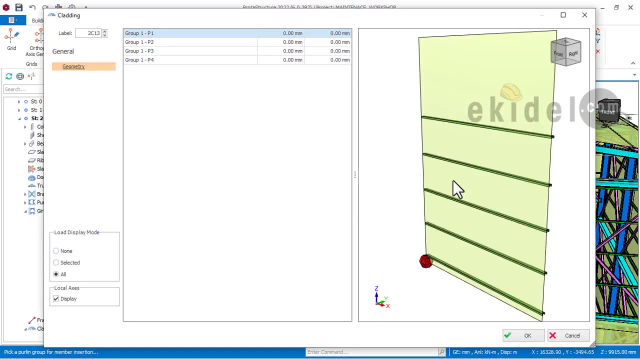 this other one here. so to create a cladding now for this place here, I'll just quickly right now and then click on the on the on the on this cycle line here now. on clicking that now, it will show me this cladding dialog box. and since I'm 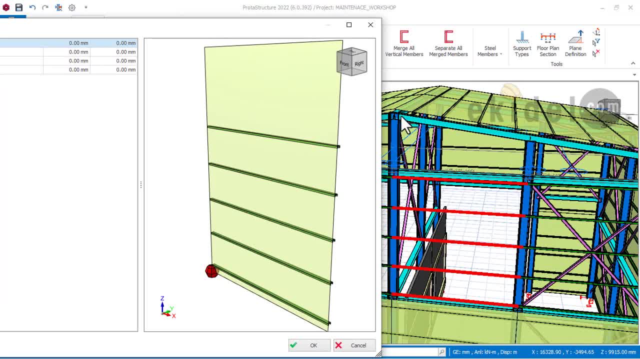 working with elevation here because I see that I want to create a cladding here and at this top here there is a slope of this steel member here, so I want my cladding to also flush with this steel slope in here. so I'll have to put in my 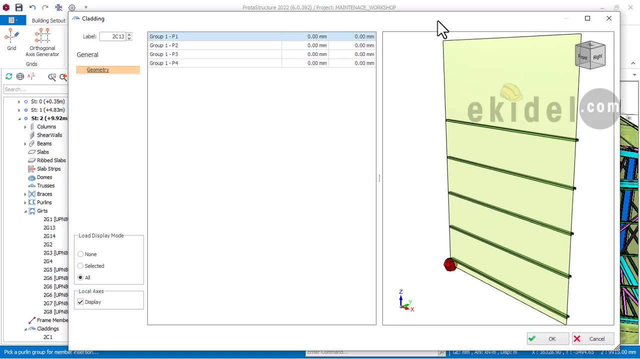 values there now and the values based on this structure, I'll have to put in the value, which i have already calculated how to put in the value and put p, p1 to be 0, p20 and p3 to now become minus um 565. you can see that. we can see that on our previous one i did um, um 656 and 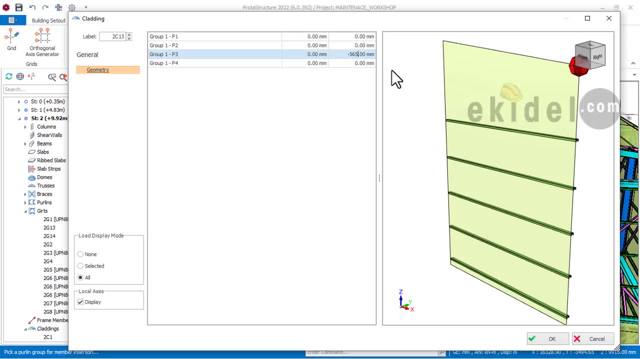 also i did minus um 200, but for this back year i have to use minus 565, because i have already done my calculations on that and i've noticed that, based on that level, i need this value for me to be able to fit in my cladding on this other side. so i'll come here right now and make my p4 to be. 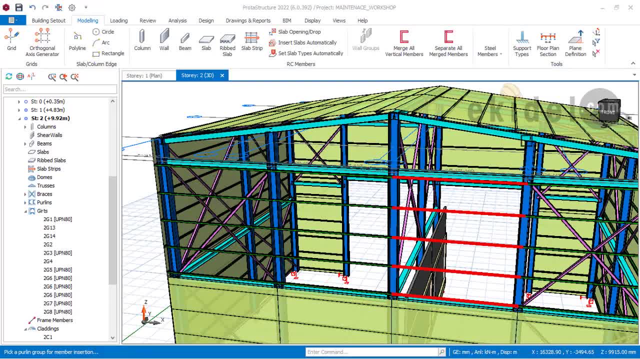 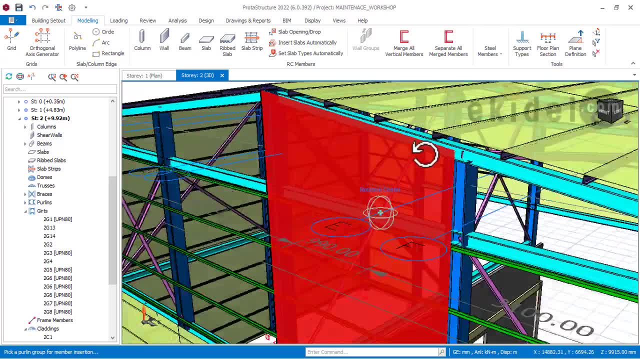 0 and now come here and then click on what: okay, automatically, right now it will just fit in. as you can see that right now it has fit in. right now, based on what i have, you can see that it is now following the same level that this team member is. okay now. i told again that cladding has what. 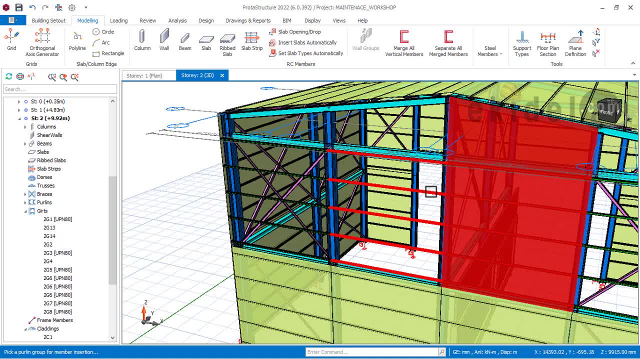 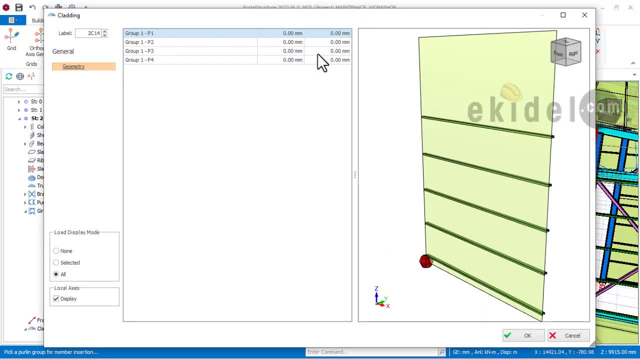 they call anti-clockwise, when you're working with cladding that has slope, okay. so this other one here, right now, to put the cladding here, i have to make it a reverse, okay so, and that reverse will just be p, p, uh, 1, 0, p 2, 0, before right now become minus um 565 and this: 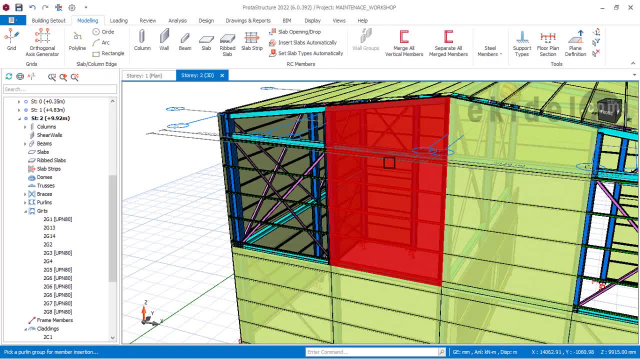 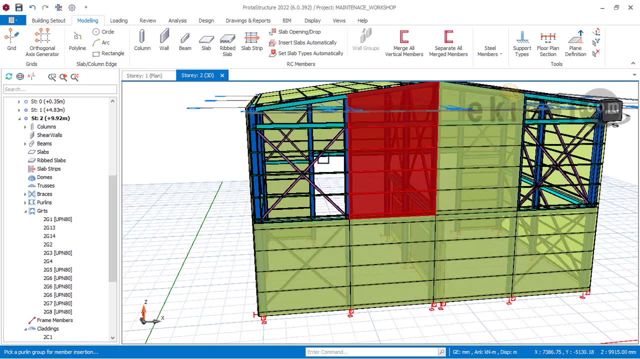 now becomes what zero, and i'll come here and say what, okay, that's fine, it will just fit in again. so right, so you can now see that we have now created another cladding for this back here. okay, that's fine. and then you can also see this other one here to not create for this other partition. 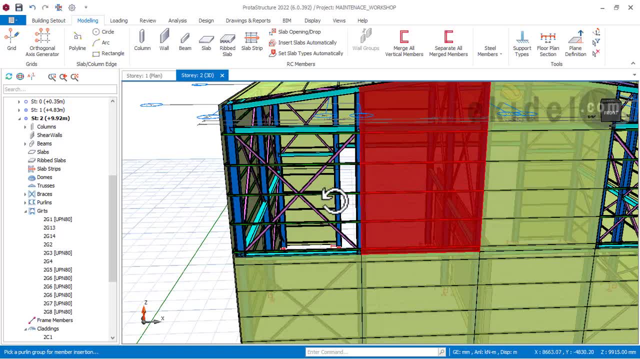 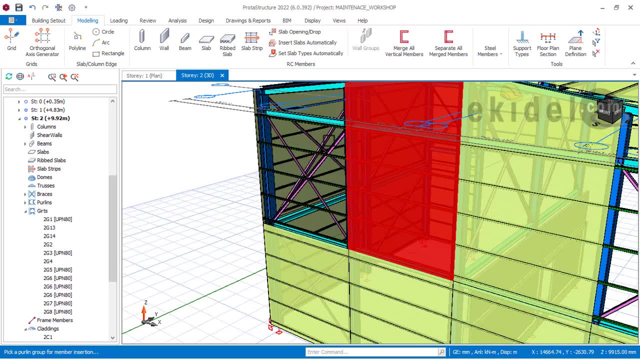 here i have to again by clicking on this other side now, by carefully clicking the cladding that that is, that is current, that is on this face for this um partition here and i'll click this now. now, once i click on it, i'll have to now come here. 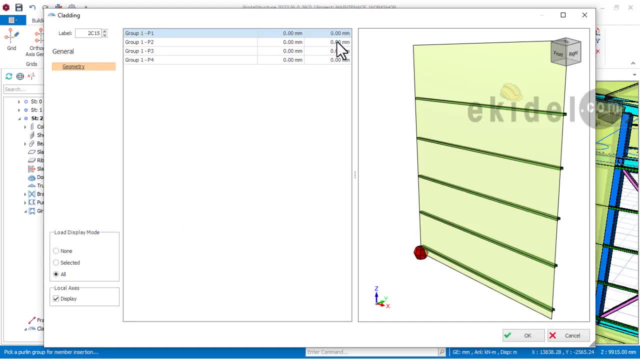 come to this place now, this p1 here is zero, p2 is zero, and then this other side here that says p3, p3 has a value of one, six, five, based on this partition, and this other one now has a value of um, um, three, five, five. and then i'll come here and then click on what, okay? and you can see that. 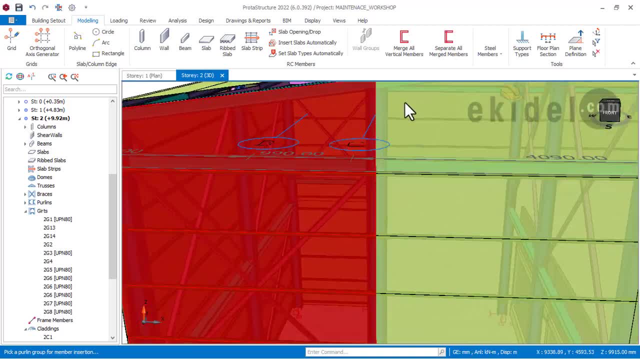 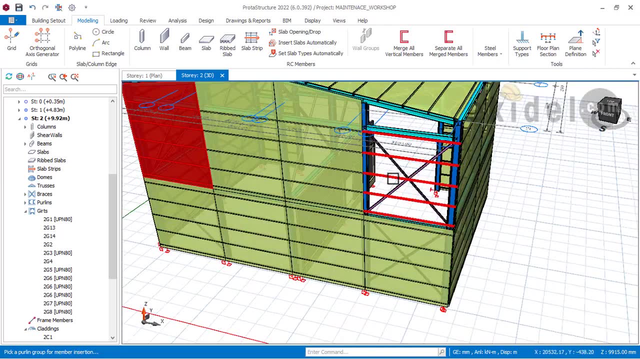 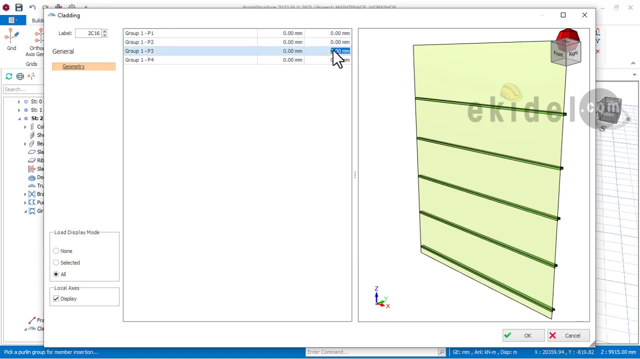 they'll just fit in. just now, you can see that they has um. it is now flushing with the slope as we have it here. okay, now again on this other side now, and then click on this place here and then come here and pp1 becomes 0p20. now p3- now we now become p3- will become um minus 355 and this one now become 1. 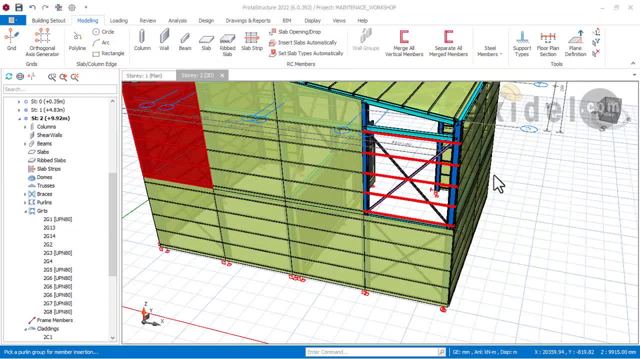 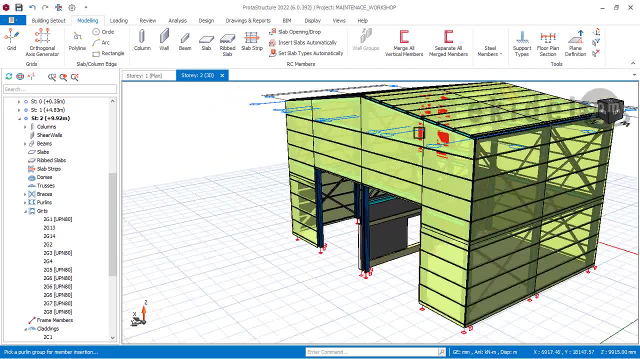 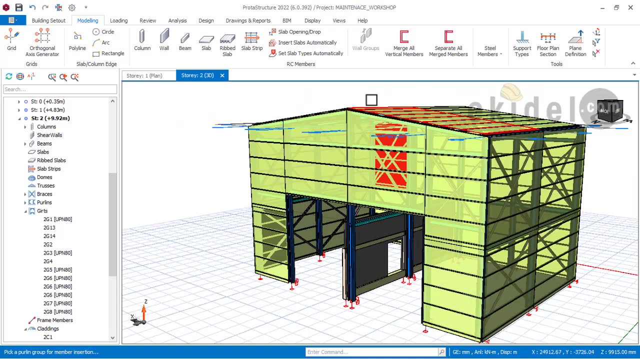 6, 5, okay, and i'll come here and then say okay, and to fit in based on this slope here. so you cannot see that we have just created um, this, our cladding based on the angle or the sloping elevation for this steel house building, as you can see that. so, basically, before the video, this was how this um. 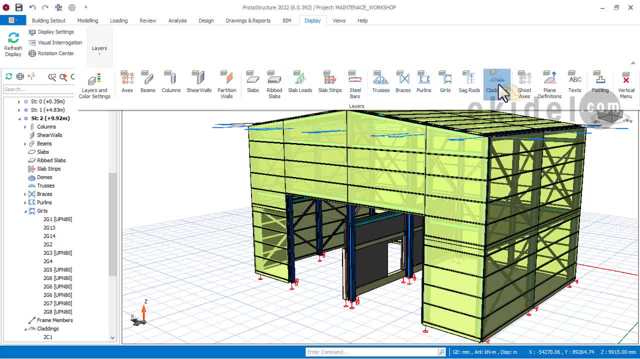 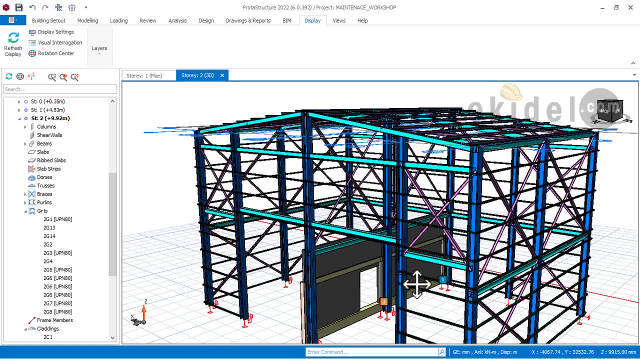 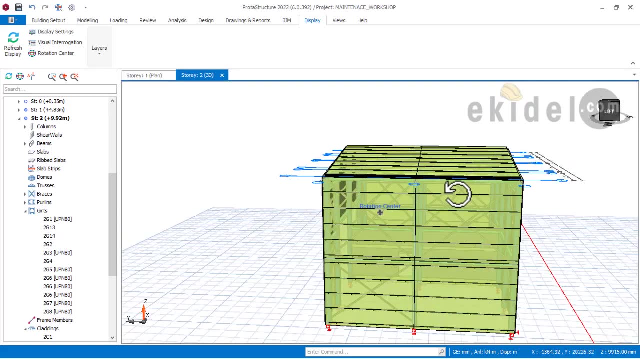 this was how this steel warehouse looked like. looks like without cladding. now, by the end of this video, as you can see, right now, we have just clotted this, our steel warehouse, with a cladding, as you can see it here. okay, so right now you cannot see our cladding. just now we have created, okay, so we considered a lot of things. 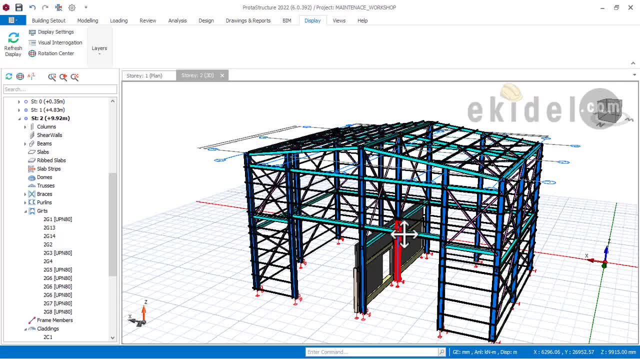 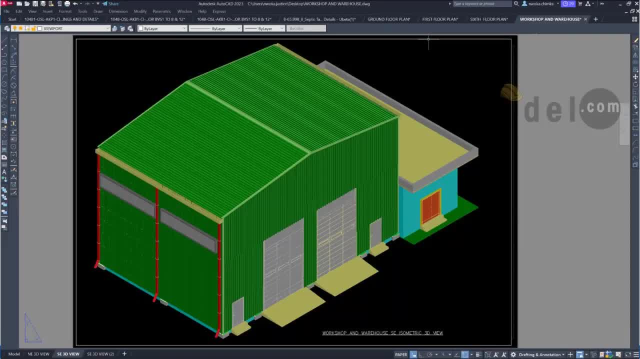 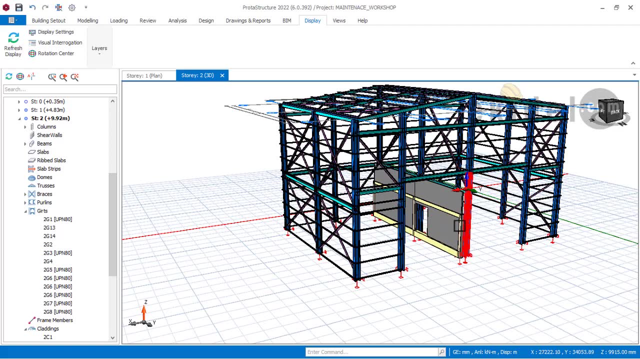 while we are doing this steel modeling, as you can see, then right now we consider a lot of things. now you can see the very picture, which is the very picture of this steel cladding. this is actually a real life project, as you can see. so we consider every um things that we are meant to consider. how 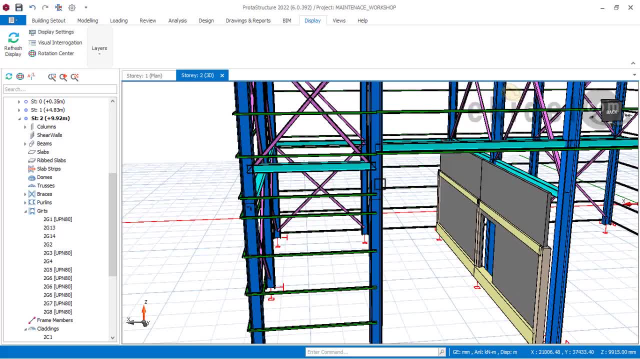 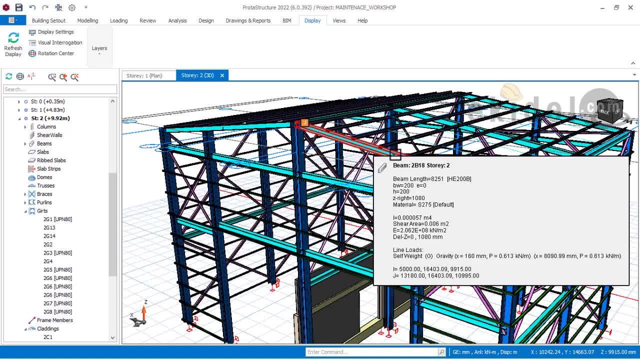 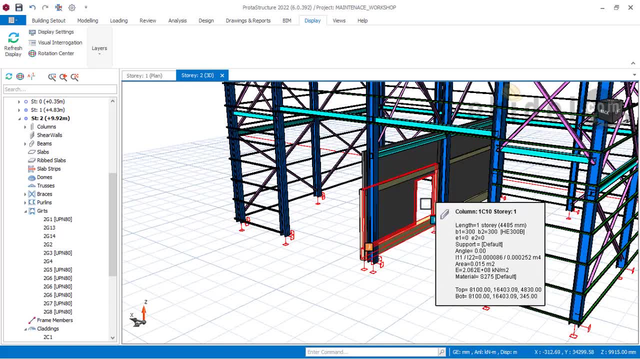 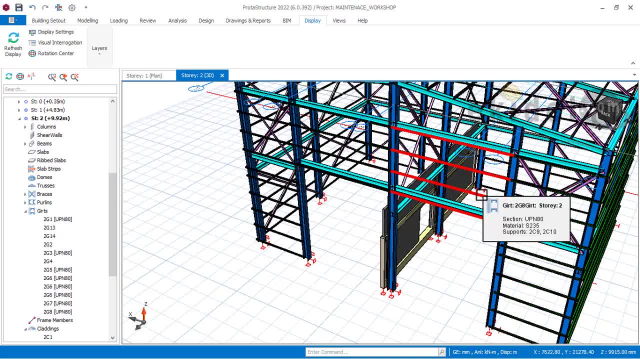 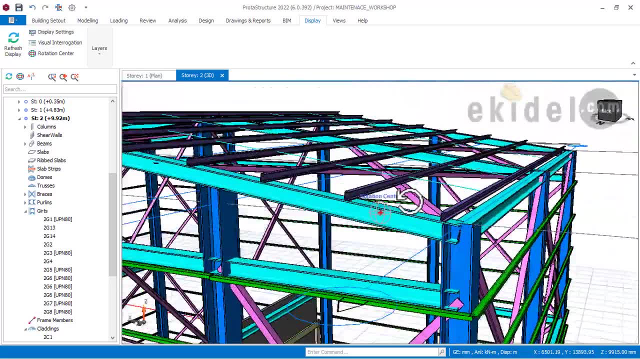 we use upn 180, as you can see that, upn 80 for our cladding, both the side cladding and the top cladding, and then for for this um, wind and brazing, we use angle ion and the angular. we use it 100 by, 100 by. 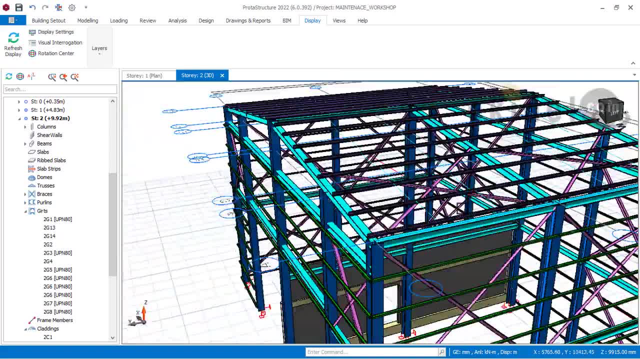 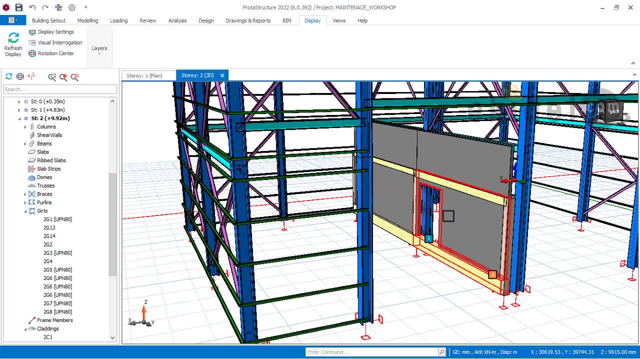 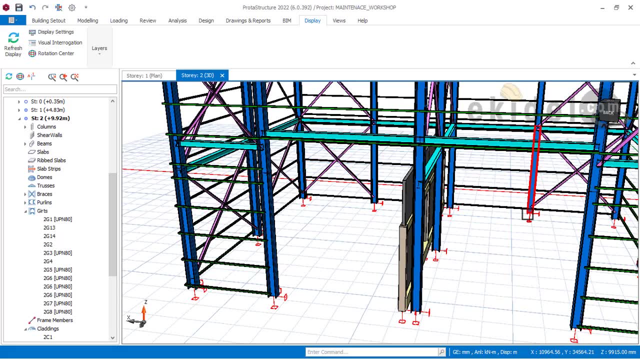 by, by eight, as you can see that. okay, so we can see how we walk through. and then this other side here, which is now um, um causing, which is now creating an entrance or let me say a demarcation between this other side of um, this um workshop, and this other side of workshop. you can see that. 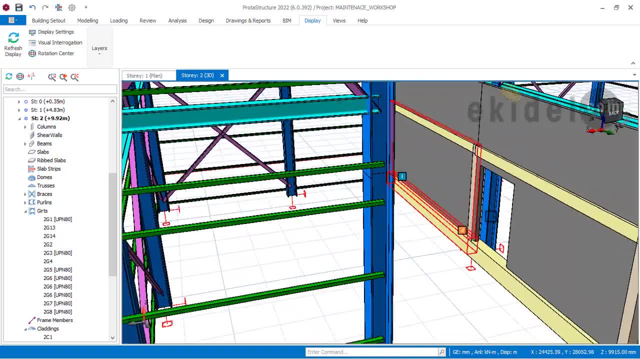 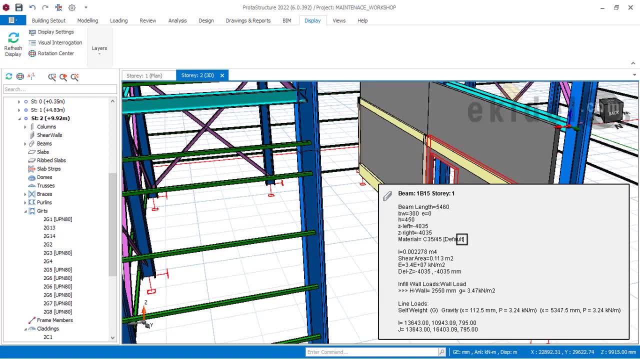 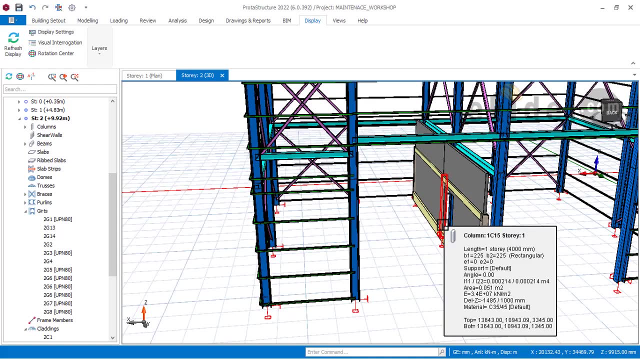 we use a concrete block wall to separate that, as you can see that. okay, so this is, this is um, this is basically how it is on the, on the, on the plan, on the build, on the, on this um steel building plan. so we are working directly with the steel building architectural plan. okay, so let's now just um go back and then close back our. 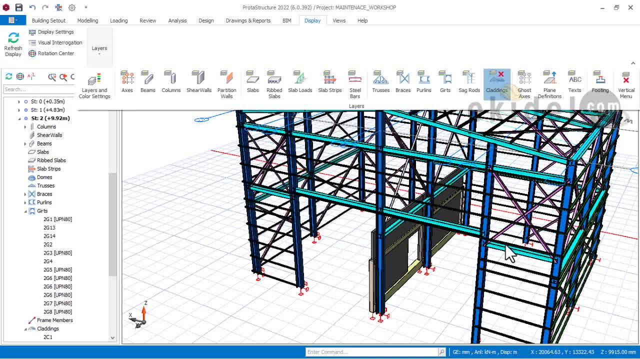 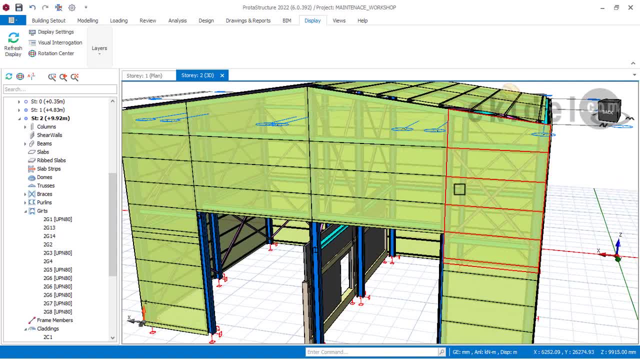 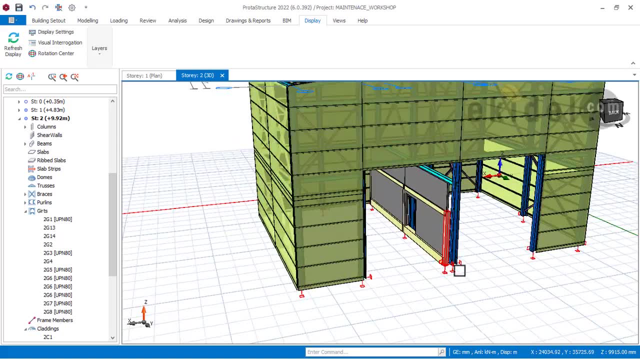 um cladding, which we have just um created. okay, so you cannot see what we have done so far, how we created this steel warehouse to this very step. so, on the next part of this maintenance, uh workshop, um steel building design, i'll be showing you how to create our concrete pedestal. now, this, the very site, or the very environment, or the very 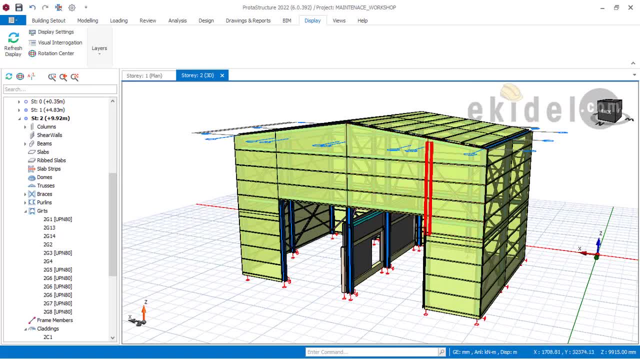 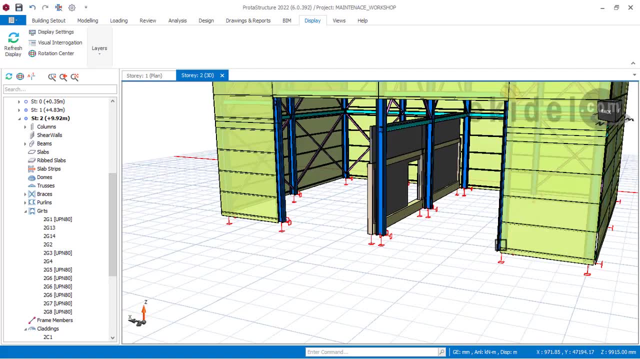 site where this workshop is going to be built has what they call water logging. so, because of that uh issue of what they call water logging, and we are going to create a very, um, big pedestal of at least one meter height so that it can, so that it can be able to protect this steel from rusting. 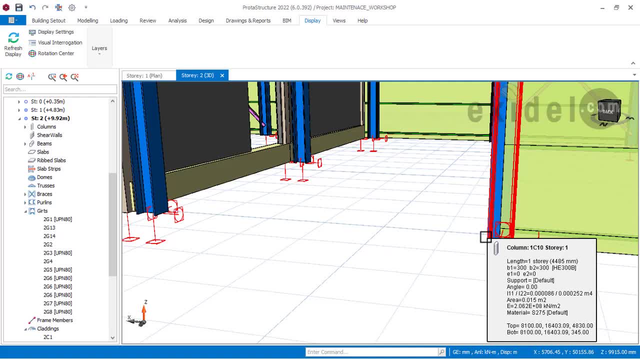 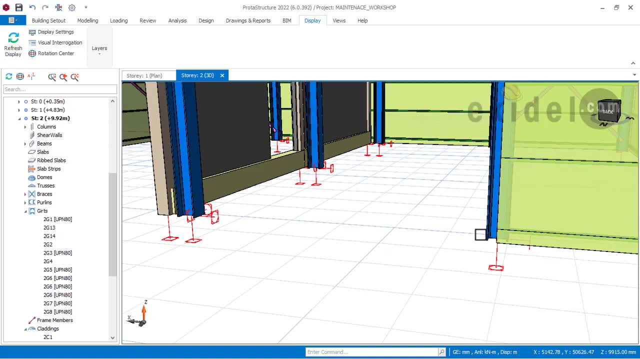 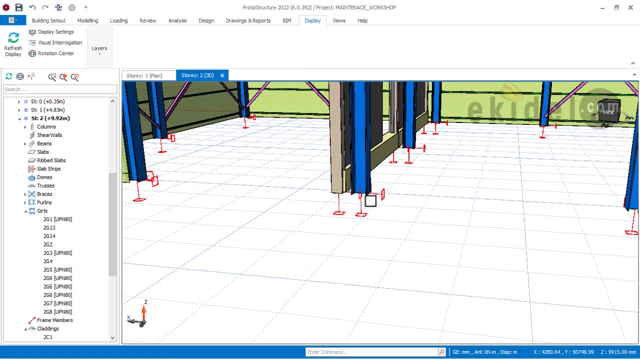 because the, because the level of water when there is, when there is a water logging on on the environment or the site, is 400. so because of that we added additional 600 to the height of our cladding to be able to protect these two members, both the boat and the base plate, from rusting. okay, now we are going to perform these. 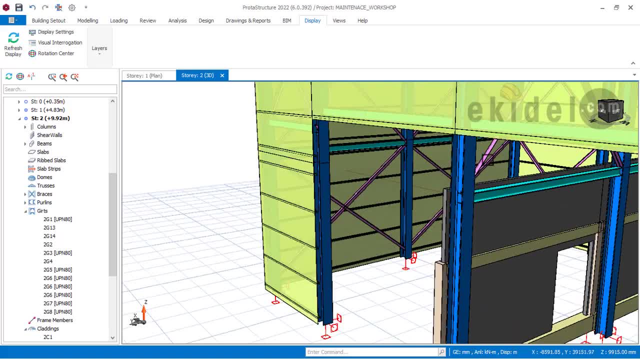 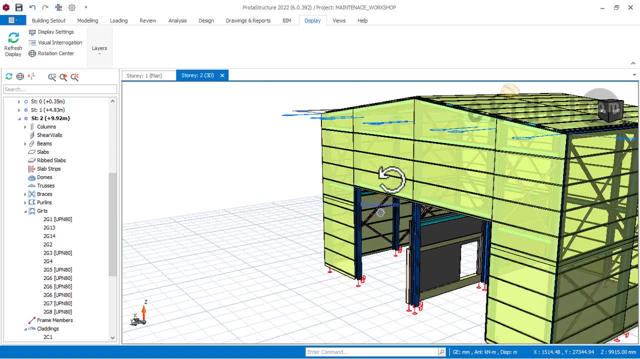 two connections for the base plate and order and also for other connections using total steel printing this tool because we are using the task, we are going to print this tool, so we are going to use that to between 22 for these three connections. okay, we have not yet done the this, uh steel. 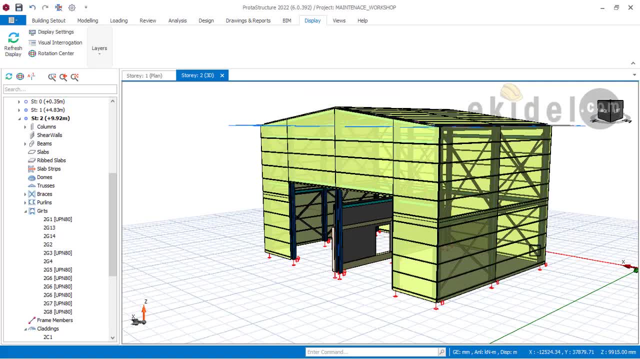 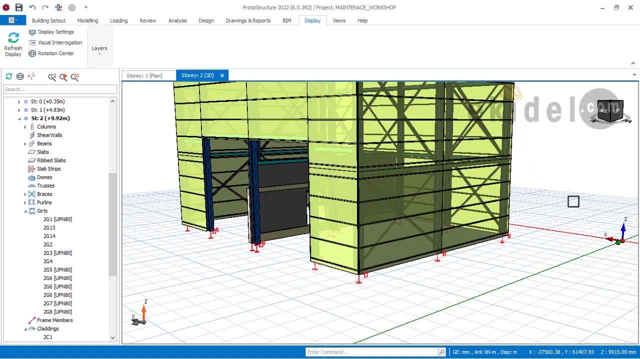 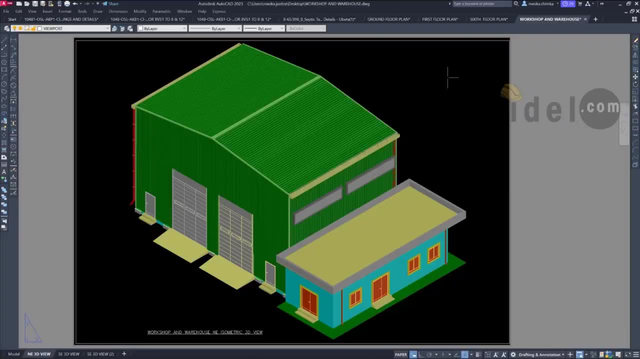 warehouse design. but we have just completed this team model, although we still have some more than two to um complete, because there is still additional smaller um um store around this place which we are going to um walk on to. as you can see it directly on the on the, on the. 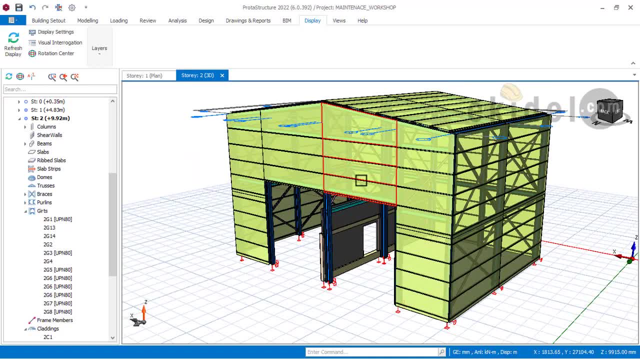 building plan. okay, so you cannot see what we have done so far. now, if this video finds it very- and it's it's a very, very helpful for you, i would say that you should click on the subscribe button and like this video and click on the video notification- um um bell, so that you don't miss. 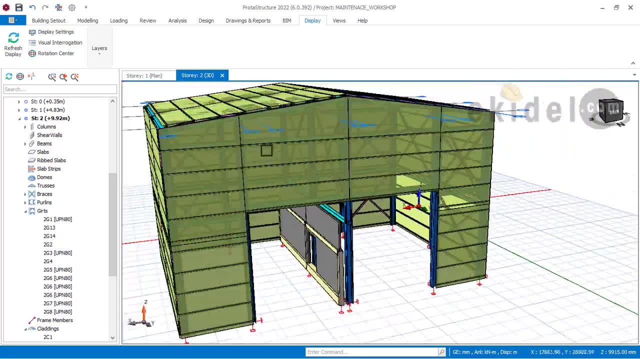 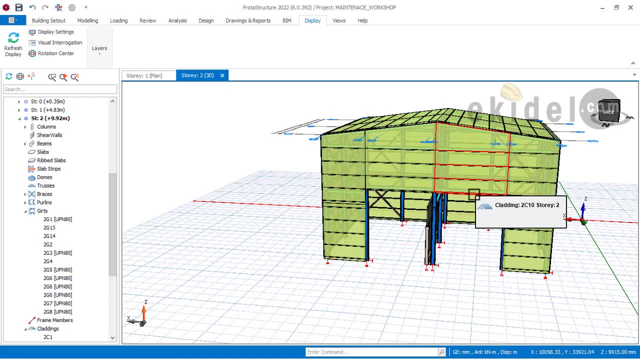 any part of this video. why we? why we are going to be uploading soon, okay. so thank you so much and god bless you. we love you. if you have any questions, so far i'll say she just drop it down on our, on, our on, on the comment section, and we have also attached our, our number. for what? whatsapp? 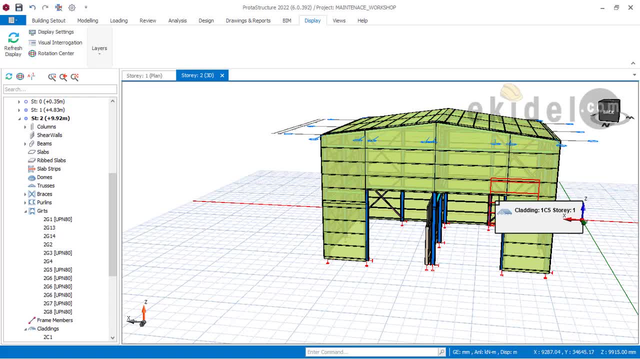 so that if maybe you have any questions, please let us know in the comment section. and we have also attached our our number for what? whatsapp, so that if maybe you want um to ask question about our, our training, our special training, which is called mentorship class, you can just quickly come and then ask questions on that. we hope we also have master.